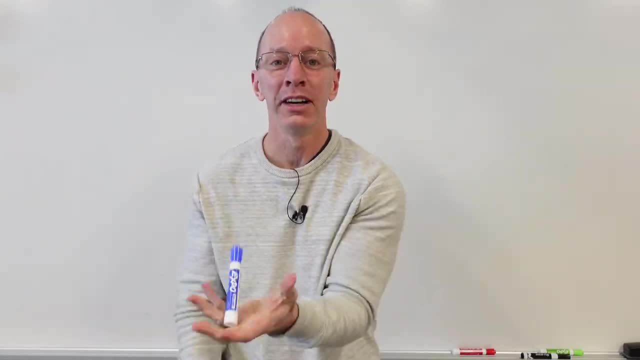 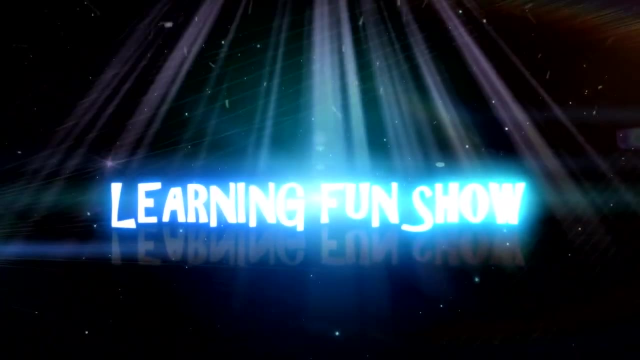 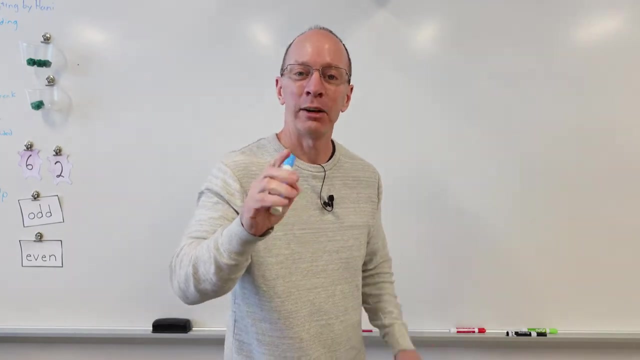 Hey, welcome to the show. Today in the show we are going to be subtracting 100 from three-digit numbers. All right, stay tuned. Hey, welcome back to the show. Today in the show we are going to be subtracting: 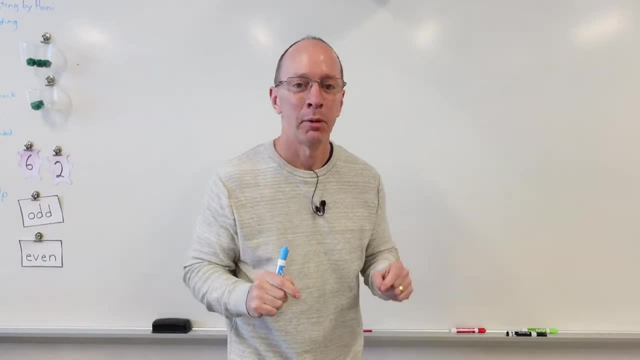 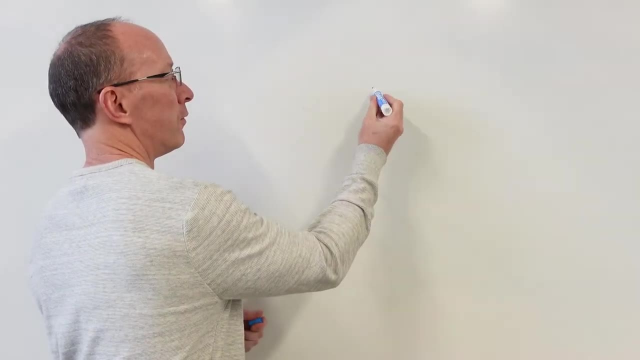 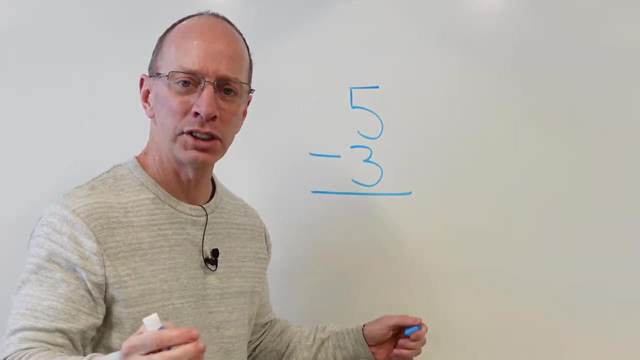 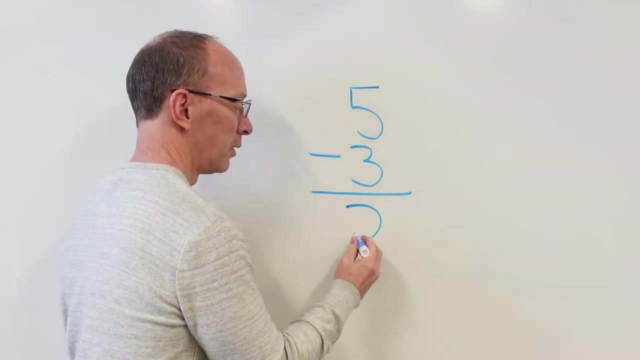 100 from a three-digit number. But before that, I want to give you a very challenging problem. Are you ready? All right, let's do it. Five minus three: Can you do that? Of course you can, because you are math ninjas. What's the answer? There you go. It is two. Five minus three is two. 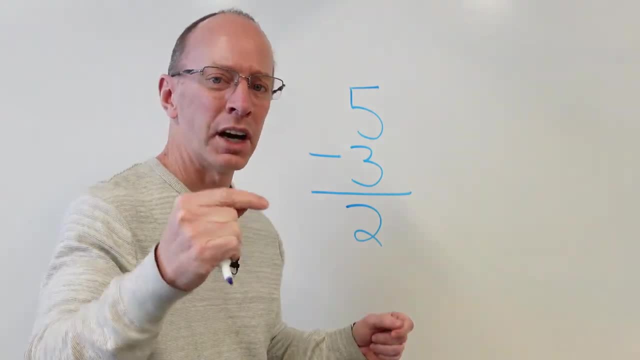 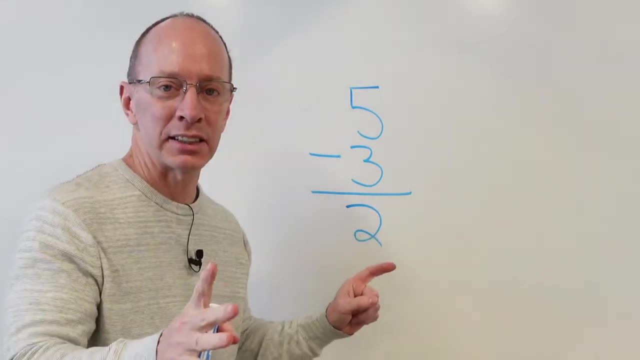 But you're saying, hey, weren't you going to be showing us how to do 100, take away 100 from a three-digit number? Yes, but we're working. We're working toward that. All right, we're working on the basics, All right. five minus three, two. 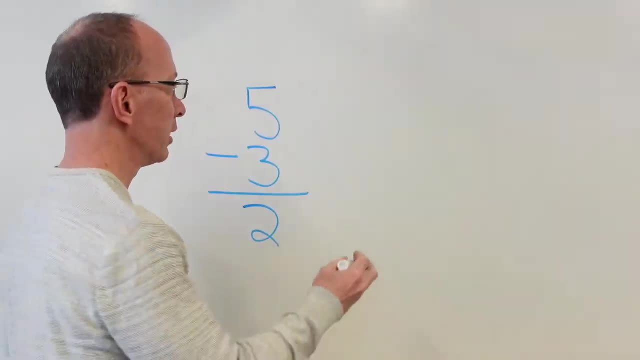 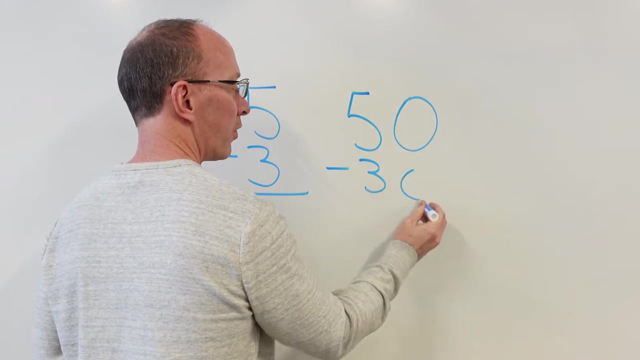 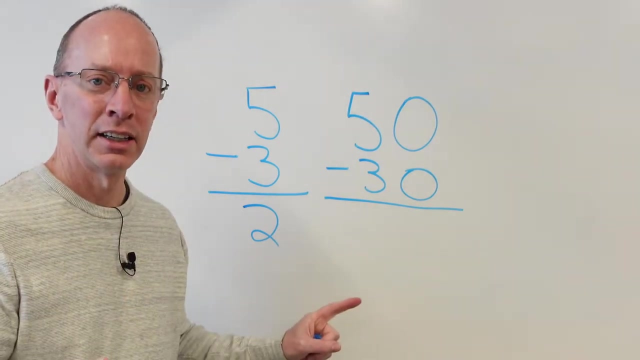 Okay, we're taking baby steps. All right, let's go on to our next problem here. Our next problem is 50 minus 30. Okay, can you do that? Take a look at that. What are your eyes first looking at? I think your eyes are first looking at that five and the three. 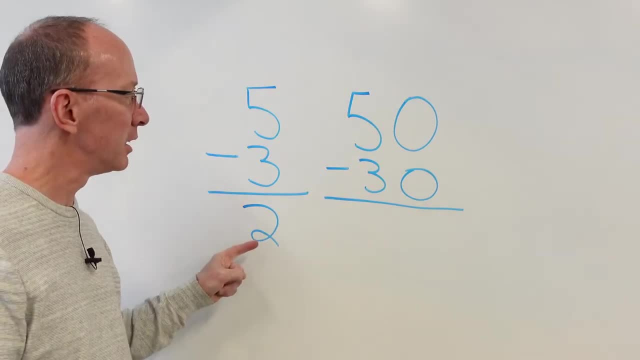 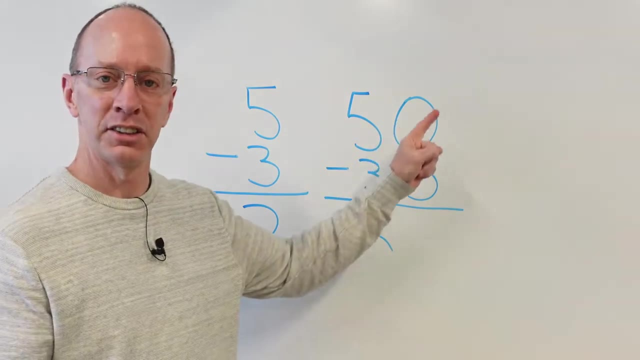 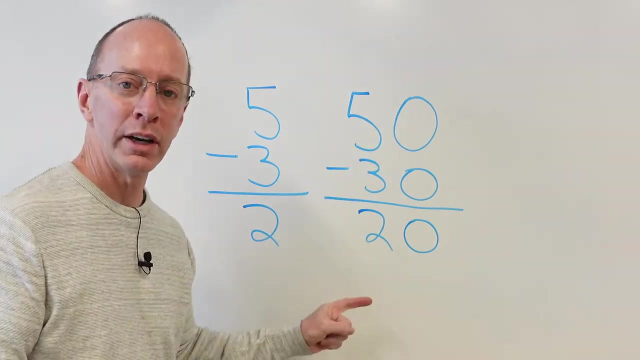 because you remember that it looks like this: five minus three. So you know that five minus three equals two, All right. and you know that zero minus zero equals zero. So 50 minus 30 equals 20.. You guys are awesome. Let's go and do the next problem. 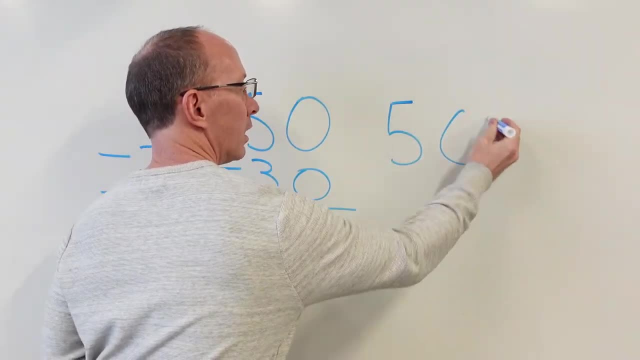 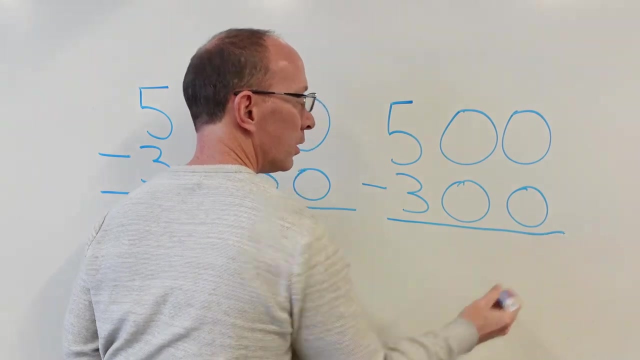 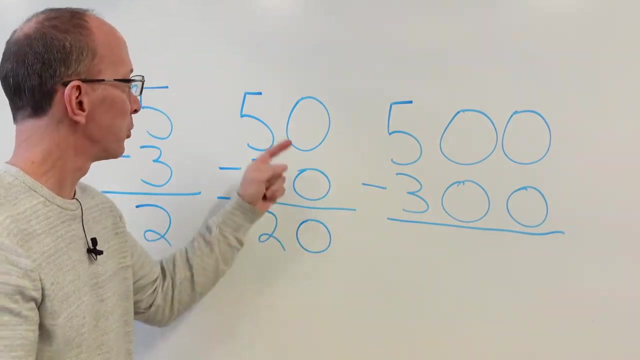 We have 500 minus 300.. 100.. All right, here's the problem. What are you first looking at? Yeah, you're looking at the five minus three, because we did that right here: Five minus three is two. Five minus three is two. 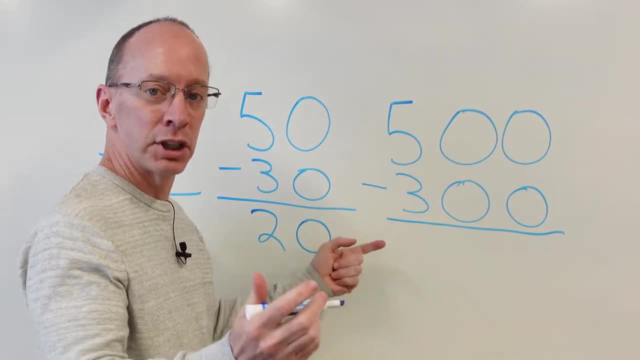 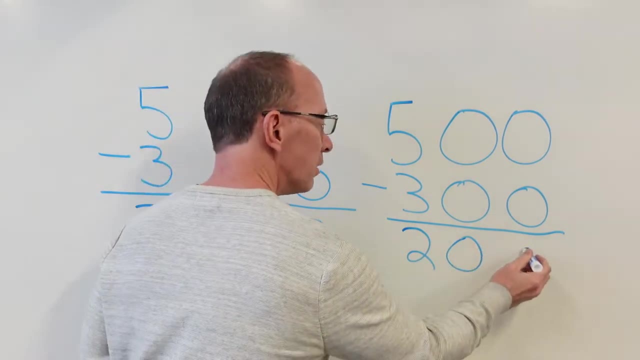 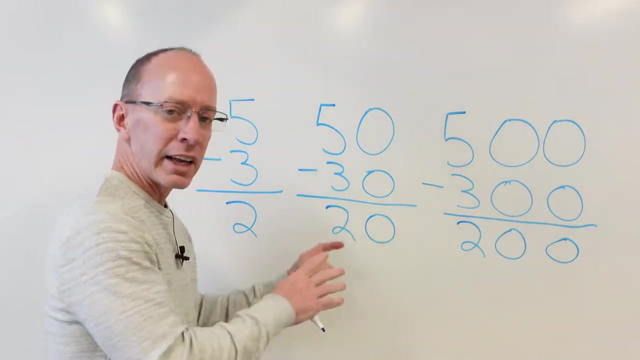 So let's go back over here: Five minus three, two Zero minus zero zero, Zero minus zero zero. Kind of catchy Zero minus zero, zero, Zero minus zero zero. All right, take a look at this. 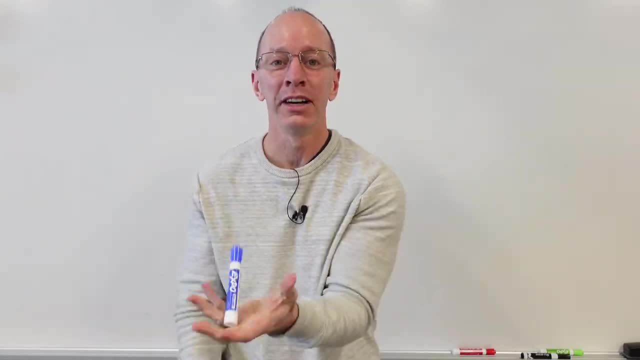 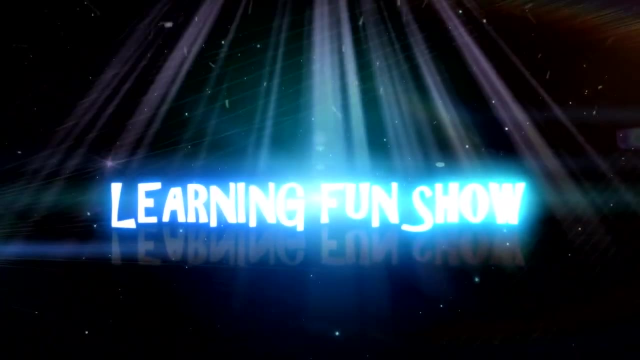 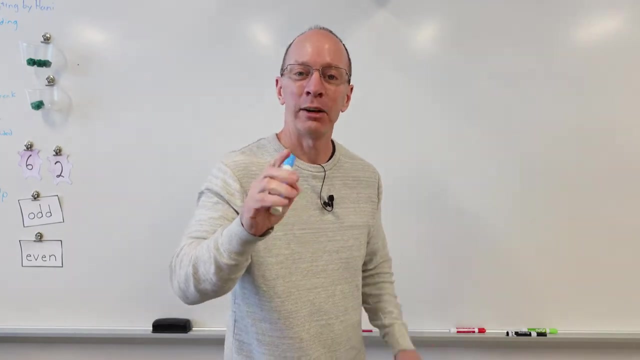 Hey, welcome to the show. Today in the show we are going to be subtracting 100 from three-digit numbers. All right, stay tuned. Hey, welcome back to the show. Today in the show we are going to be subtracting: 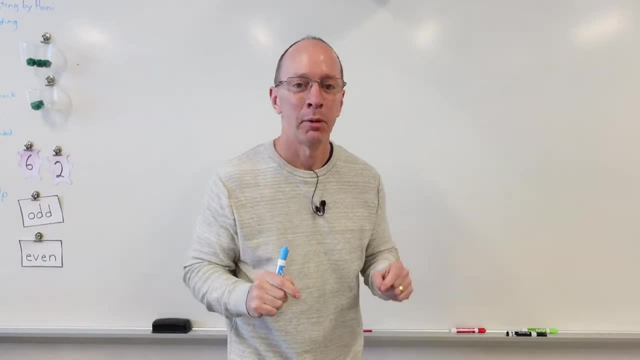 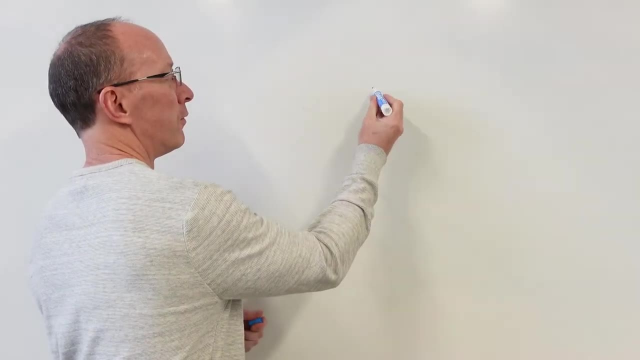 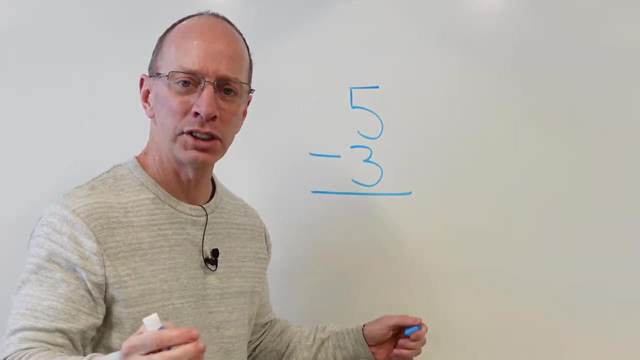 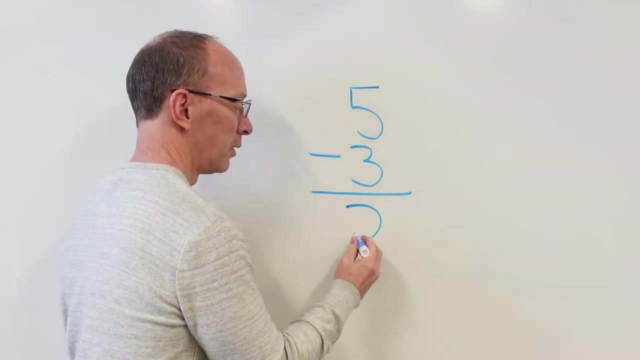 100 from a three-digit number. But before that, I want to give you a very challenging problem. Are you ready? All right, let's do it. Five minus three: Can you do that? Of course you can, because you are math ninjas. What's the answer? There you go. It is two. Five minus three is two. 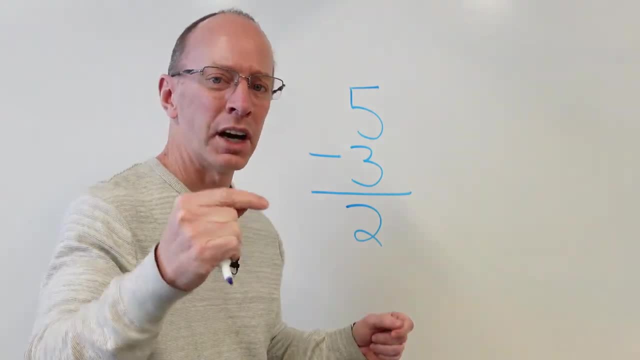 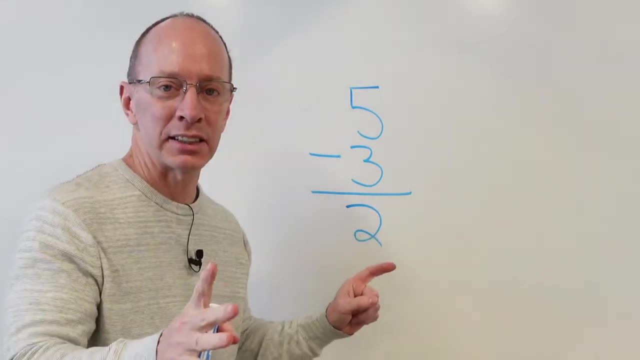 But you're saying, hey, weren't you going to be showing us how to do 100, take away 100 from a three-digit number? Yes, but we're working. We're working toward that. All right, we're working on the basics, All right. five minus three, two. 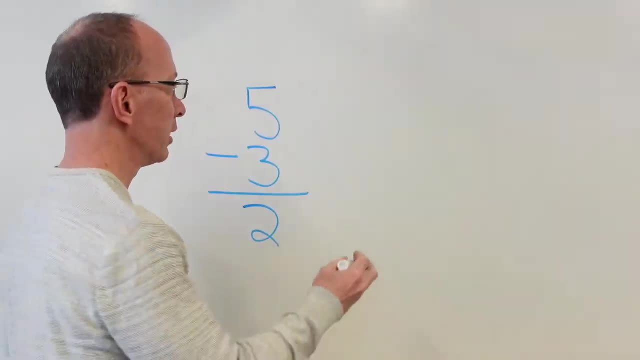 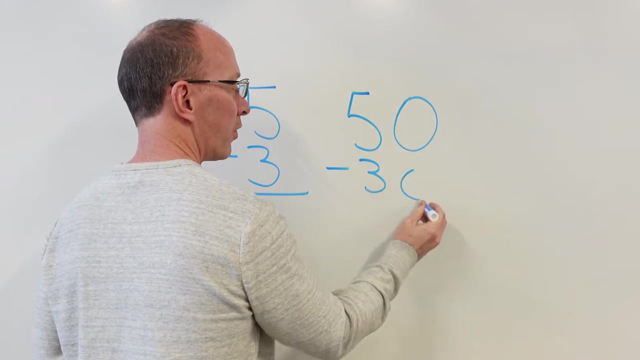 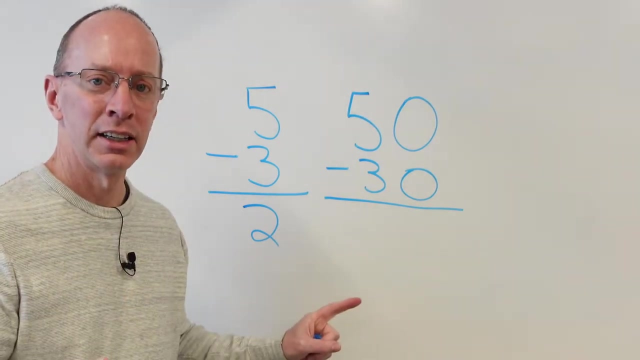 Okay, we're taking baby steps. All right, let's go on to our next problem here. Our next problem is 50 minus 30. Okay, can you do that? Take a look at that. What are your eyes first looking at? I think your eyes are first looking at that five and the three. 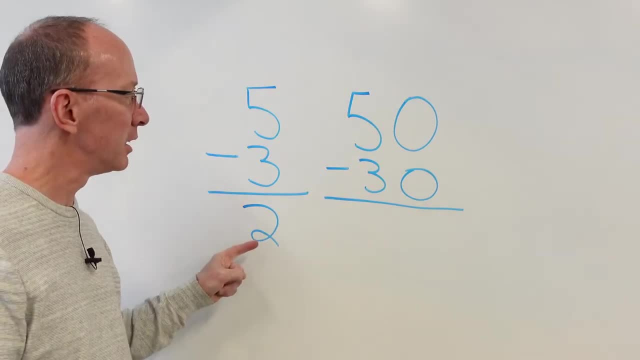 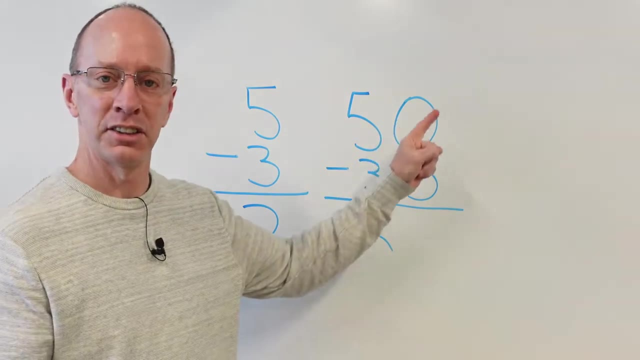 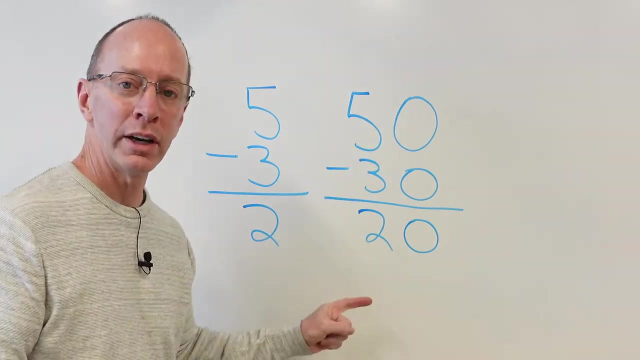 because you remember that it looks like this: five minus three. So you know that five minus three equals two, All right. and you know that zero minus zero equals zero. So 50 minus 30 equals 20.. You guys are awesome. Let's go and do the next problem. 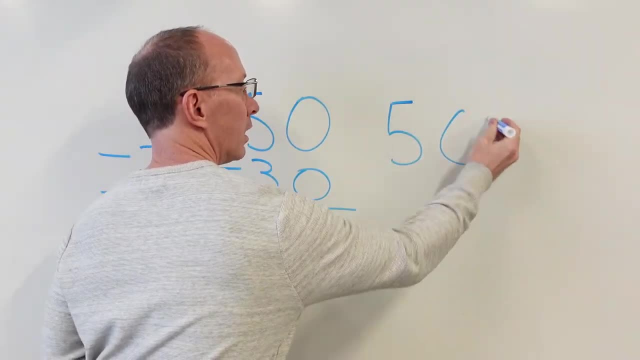 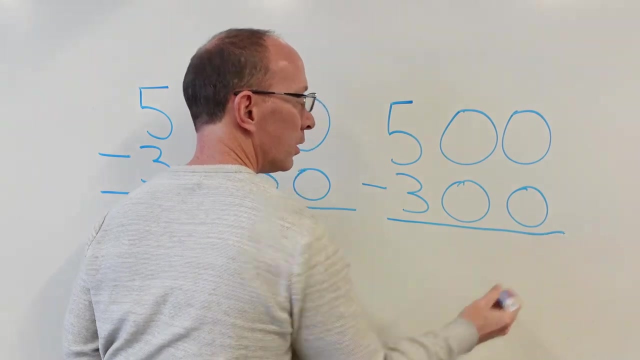 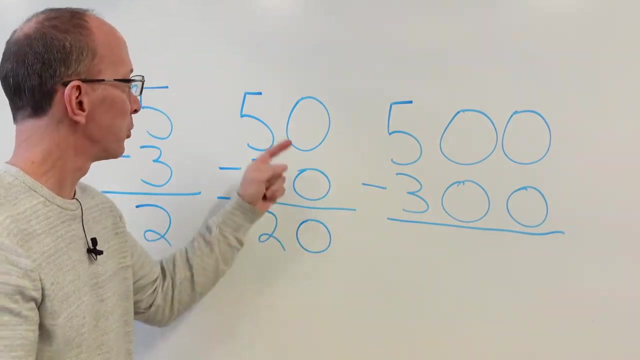 We have 500 minus 300.. 100.. All right, here's the problem. What are you first looking at? Yeah, you're looking at the five minus three, because we did that right here: Five minus three is two. Five minus three is two. 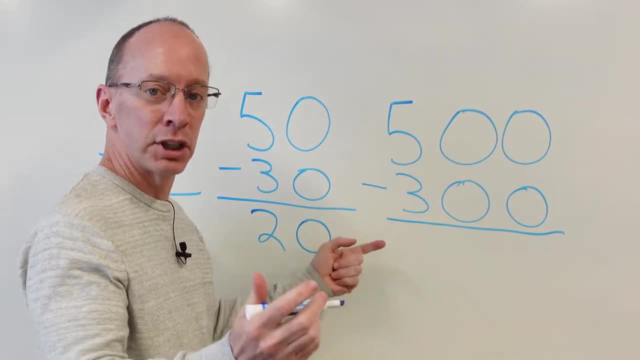 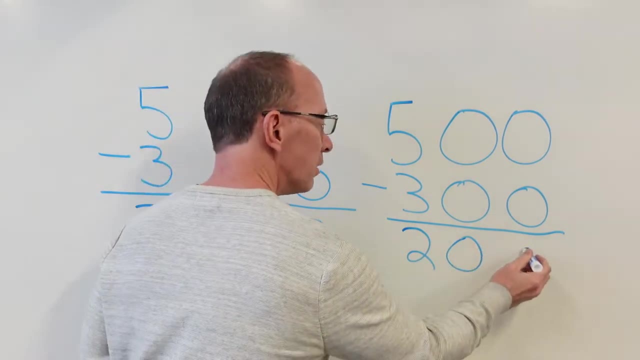 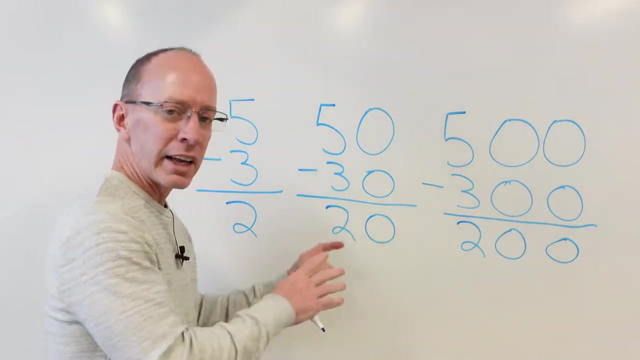 So let's go back over here: Five minus three, two Zero minus zero zero, Zero minus zero zero. Kind of catchy Zero minus zero, zero, Zero minus zero zero. All right, take a look at this. 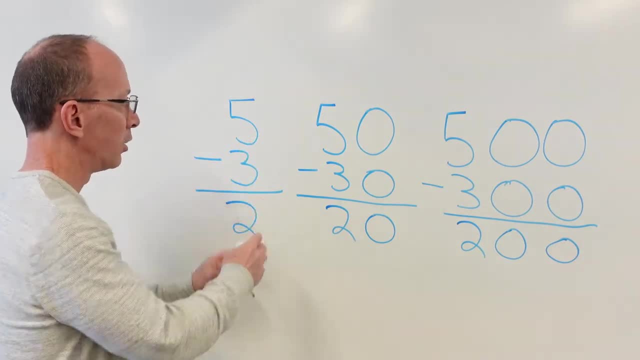 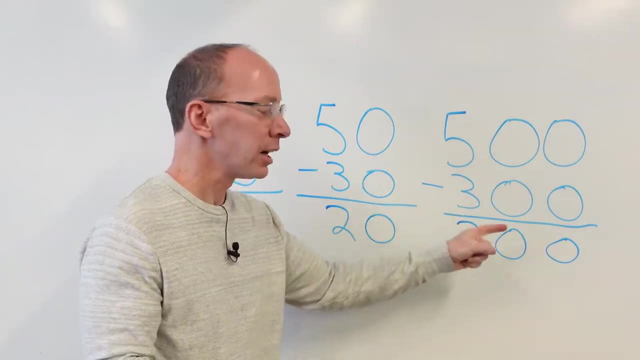 Your eyes are first looking at the five minus three. All right, let's go back over here: Five minus three. When we did 50 minus 30, your eyes looked at the five minus three and you put a two. When you did 500 minus 300, your eyes looked at the five and the three, and that was two. 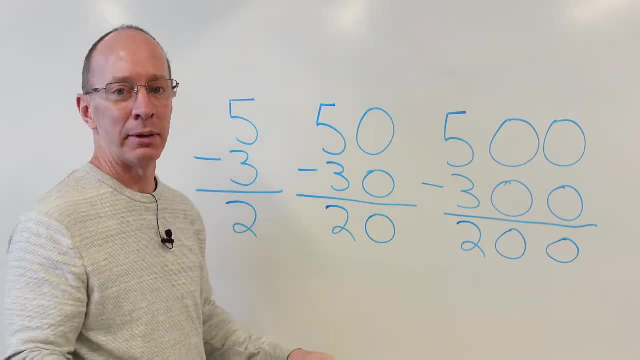 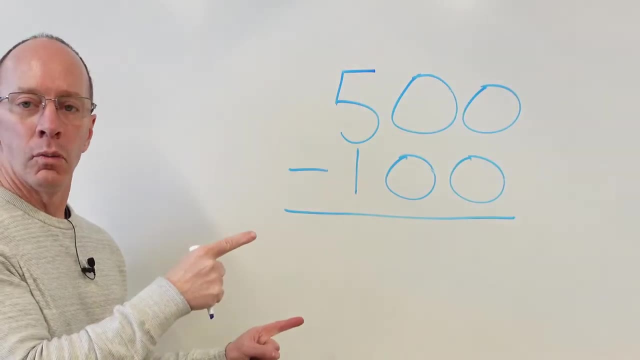 All right, see, You took baby steps and now you're becoming a master math ninja. All right, ready to go on to the next problem? Yeah, let's do it. Yeah, Whoa, here we go. Okay, right away, when you're taking a look at this problem here? 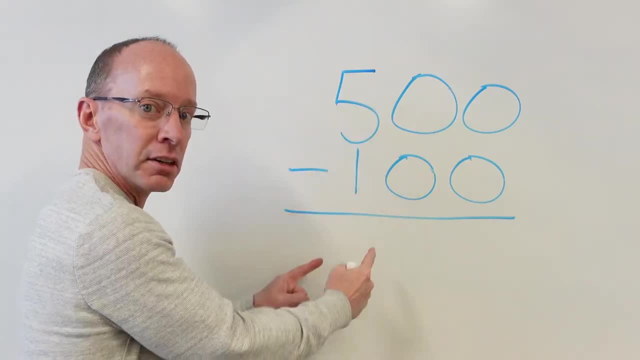 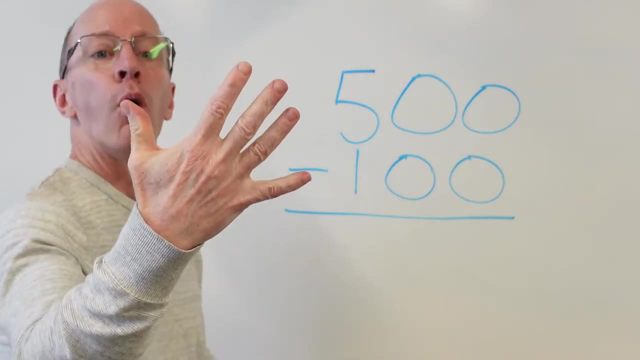 what are you looking at? You're looking at this, aren't you Right? Your eyeballs were looking at this: five minus one. What is five minus one? Five? take away one Bam, you got four. All right, uno dos tres cuatro. 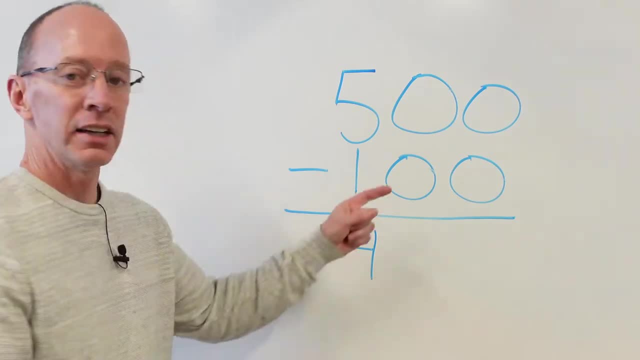 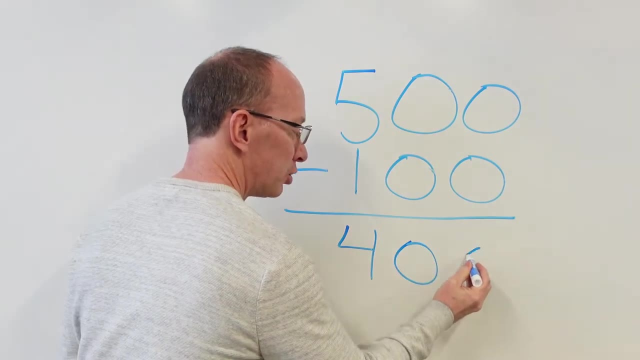 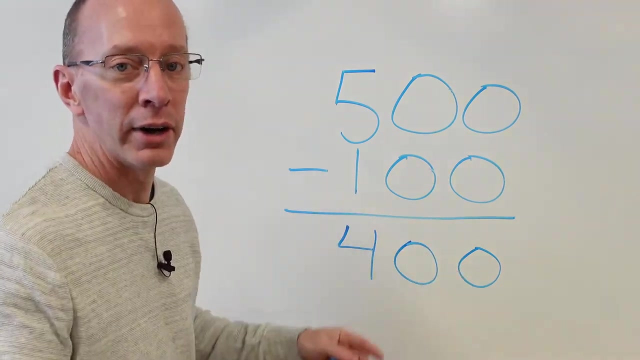 Five minus one is four. Then zero minus zero, You got zero. take away another zero. There's nothing right there. Zero minus zero. Drop that zero down. drop the other zero down. 500 minus 100 equals 400.. All right, ready to do the next problem? Yeah, let's do it. Yeah, Boom, right away. Hey. 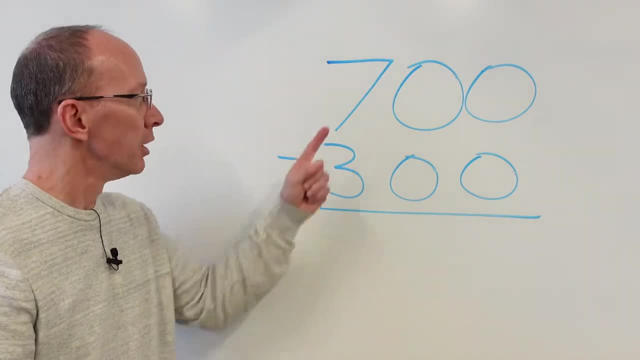 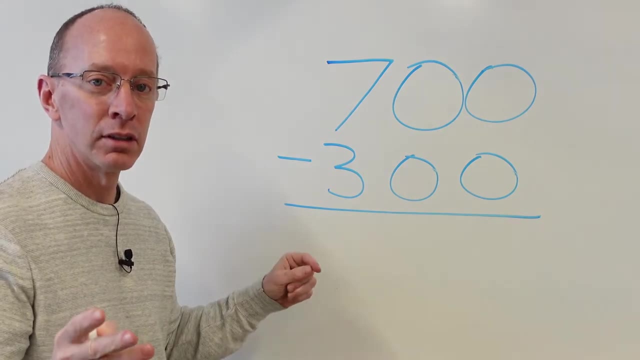 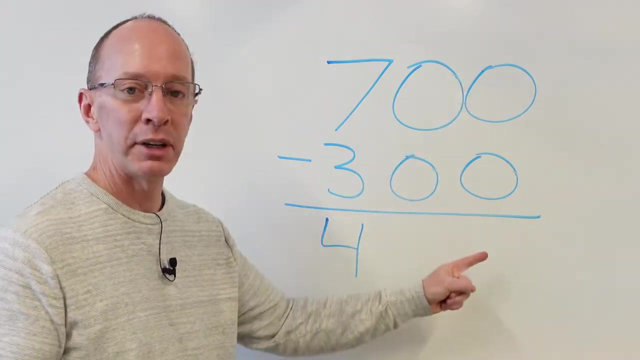 where's your eyeballs going to? What are you looking at? Yeah, you're looking right in here, aren't you? You're looking at seven minus three. Seven minus three equals. You got it four. Seven minus three equals four. Then you just subtract the zeros, Drop it down, Drop it. 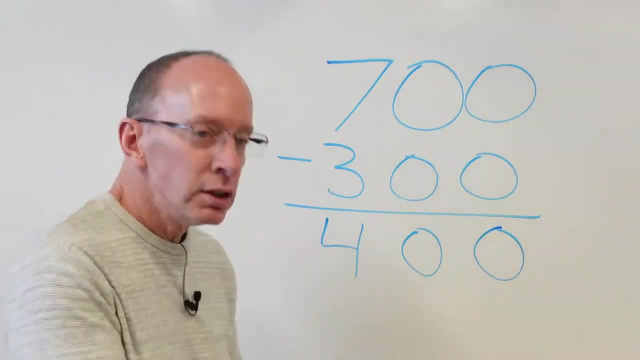 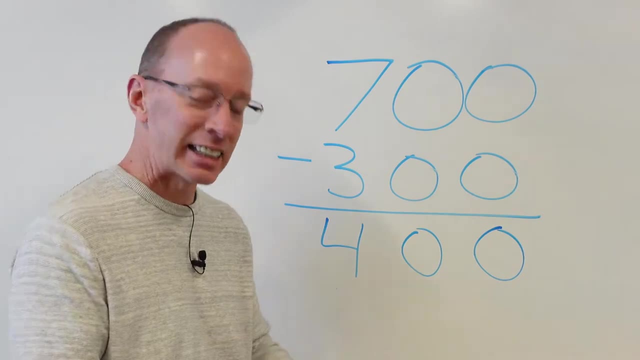 Drop it, Drop the zeros, Drop it, Drop it, Drop the zeros. Okay, Yeah, I hear your teacher. She's saying, or he or she is saying come on, hurry up with the lesson. All right, So, but basically, this is really easy cheesy lemon. 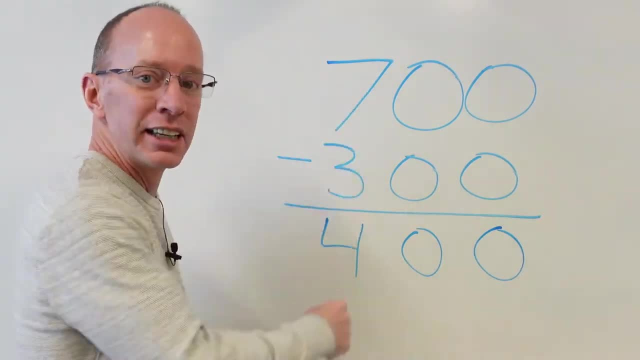 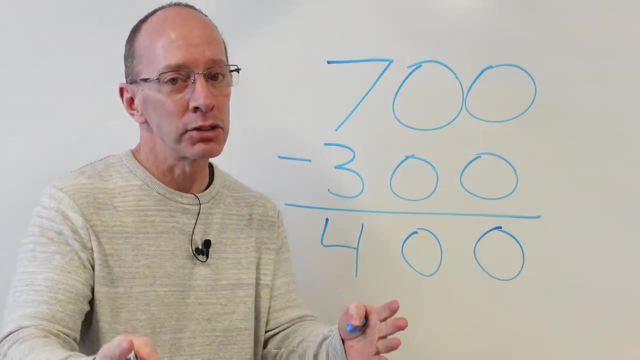 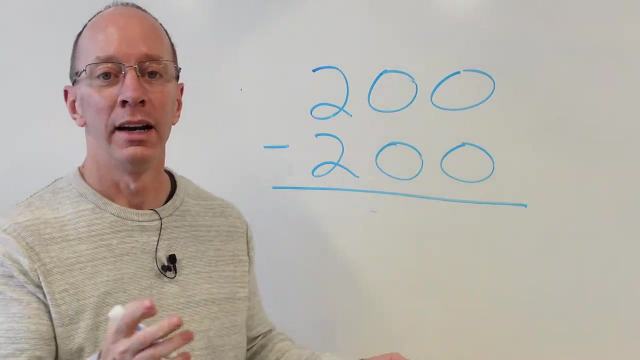 squeezy. You take a look at the numbers that you can subtract right away when you're dealing with subtracting hundreds from a three-digit number Also works with a two-digit number. But hey, this is super fun, Let's do another one. Yeah, let's do it. Yeah, Boom, Whoa, All right. 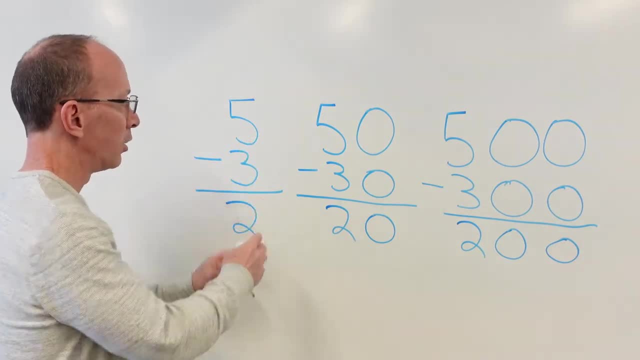 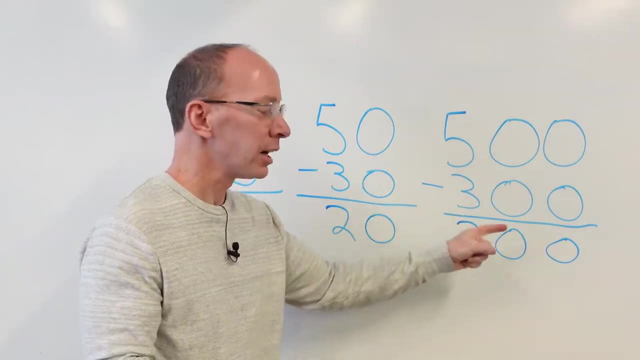 Your eyes are first looking at the five minus three. All right, let's go back over here: Five minus three. When we did 50 minus 30, your eyes looked at the five minus three and you put a two. When you did 500 minus 300, your eyes looked at the five and the three, and that was two. 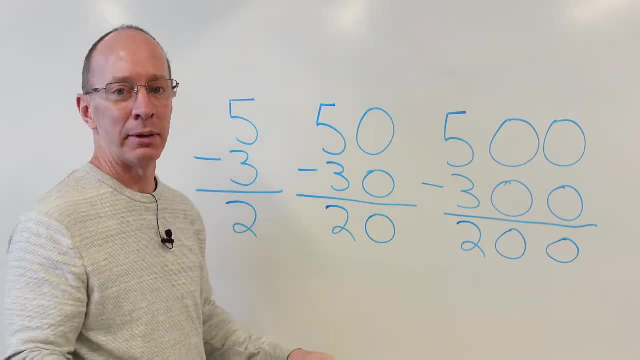 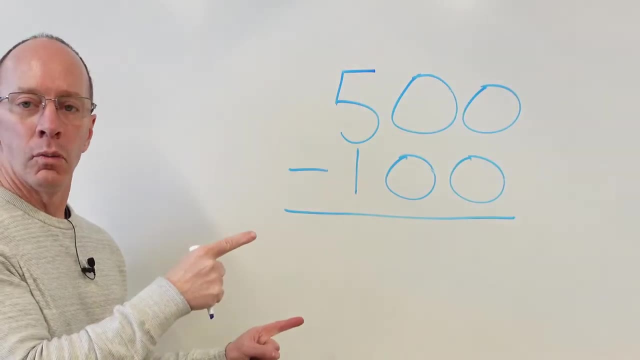 All right, see, You took baby steps and now you're becoming a master math ninja. All right, ready to go on to the next problem? Yeah, let's do it. Yeah, Whoa, here we go. Okay, right away, when you're taking a look at this problem here? 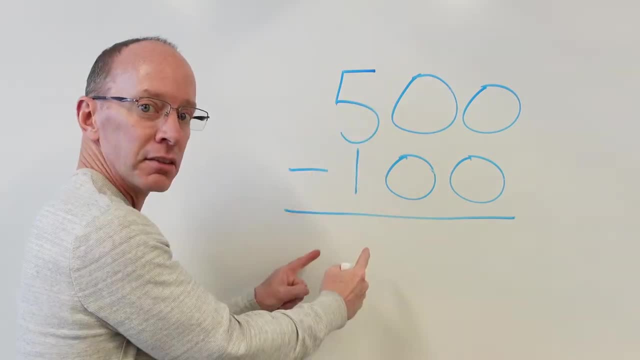 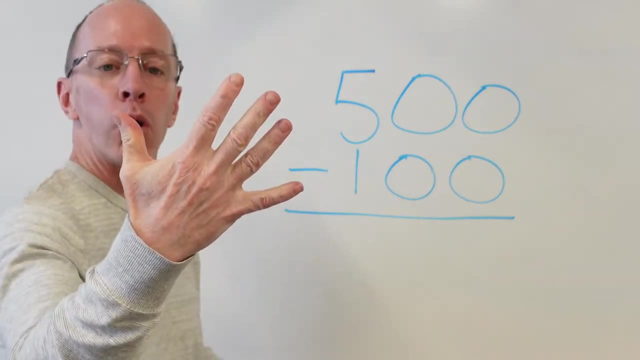 what are you looking at? You're looking at this, aren't you Right? Your eyeballs were looking at this: five minus one. What is five minus one? Five? take away one Bam, you got four. All right, uno dos tres cuatro. 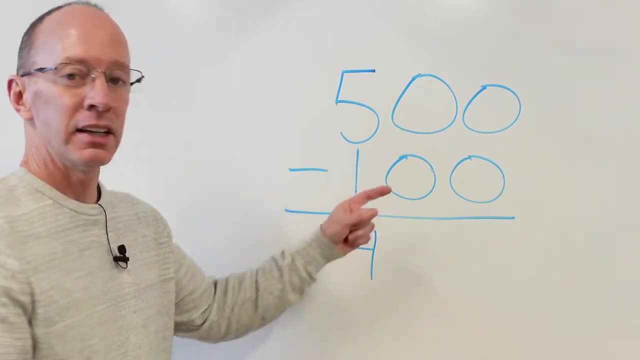 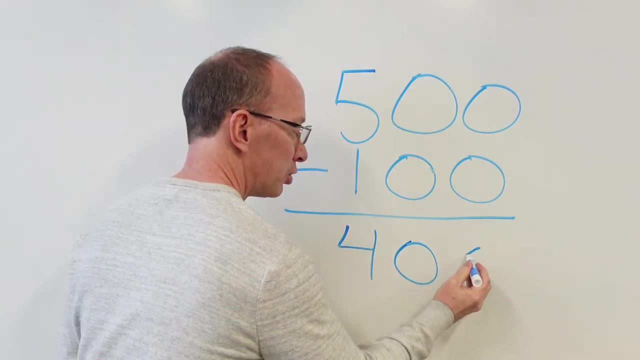 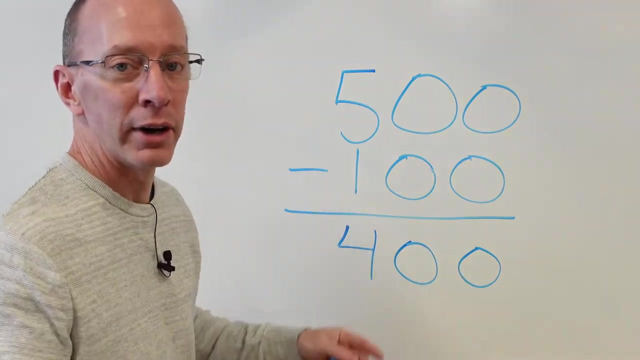 Five minus one is four. Then zero minus zero, You got zero. take away another zero. There's nothing right there. Zero minus zero. Drop that zero down. drop the other zero down. 500 minus 100 equals 400.. All right, ready to do the next problem? Yeah, let's do it. Yeah, Boom, right away. 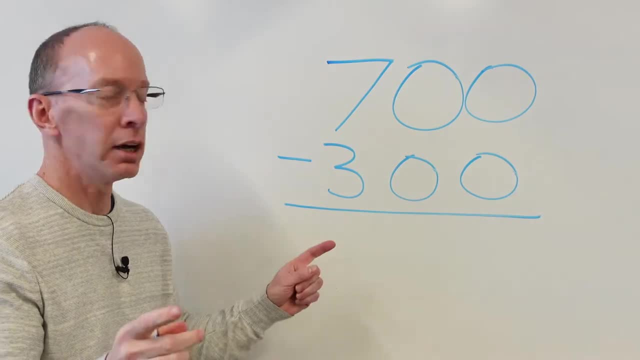 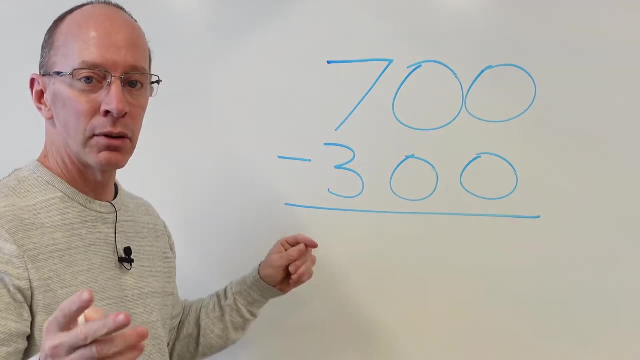 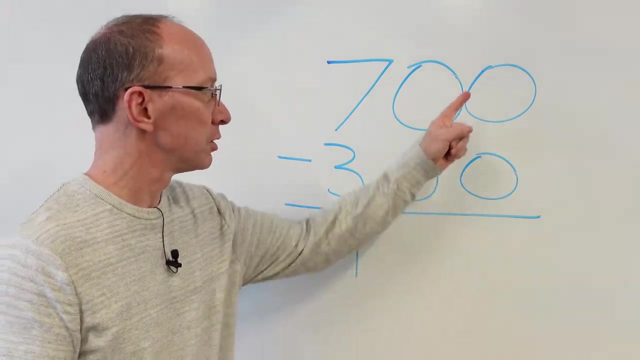 Hey, where's your eyeballs going to? What are you looking at? Yeah, you're looking right in here, aren't you? You're looking at seven minus three. Seven minus three equals. you got it: four. Seven minus three equals four. Then you just subtract the zeros, Drop it down, Drop it, Drop it, Drop the. 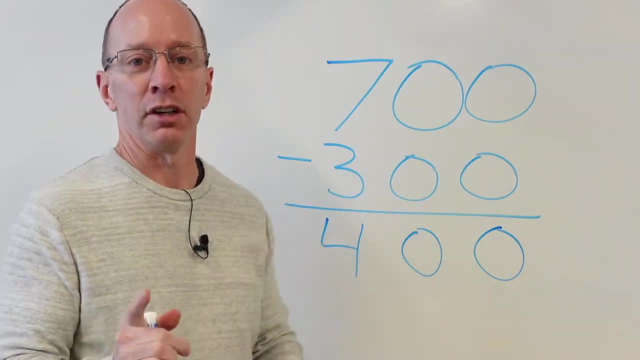 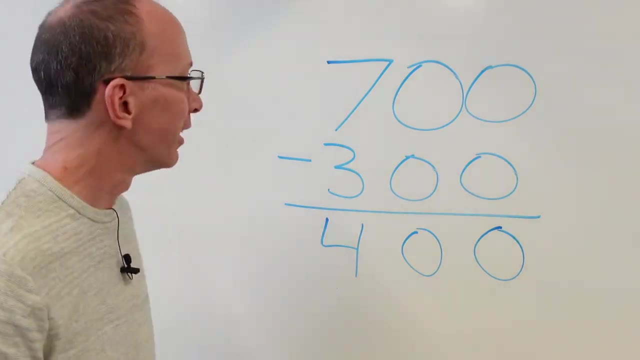 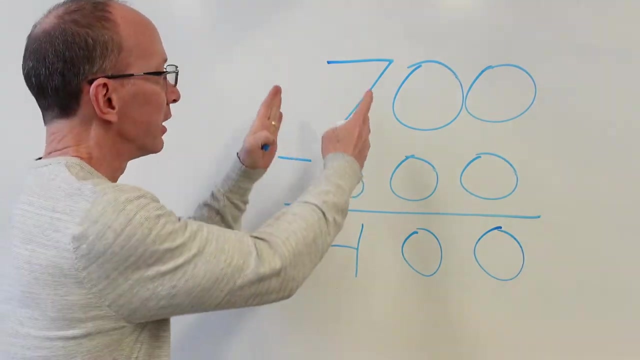 zeros, Drop it, Drop it, Drop the zeros. Okay, Yeah, I hear your teacher. She's saying he or she is saying come on, hurry up with the lesson. All right, So, but basically, this is really easy: cheesy, lemon, squeezy. You take a look at the numbers that you can subtract right away. 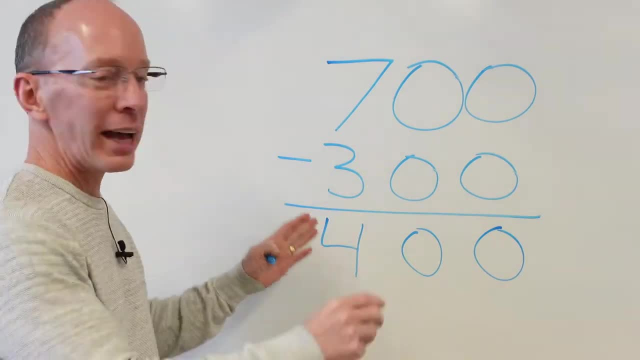 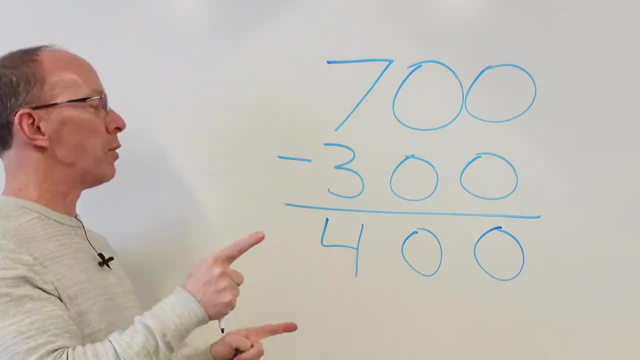 when you're dealing with subtracting hundreds from a three-digit number Also works with a two-digit number. But hey, this is super fun, Let's do another one. Yeah, let's do it. Yeah, Boom, Whoa, All right, All right, Right away I can tell you math. ninjas, you are looking at this. 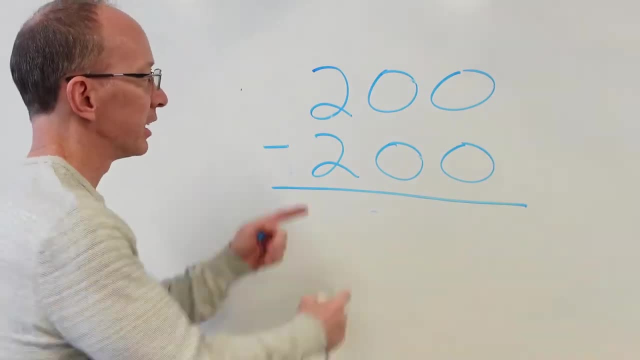 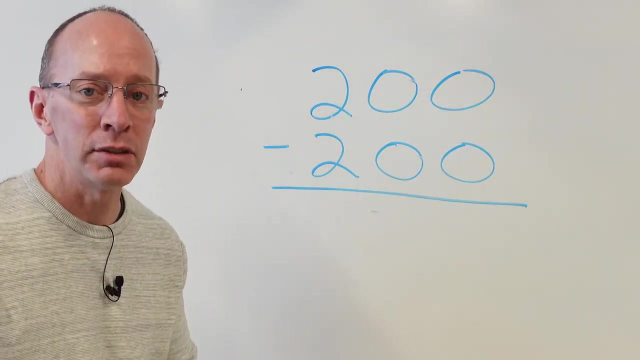 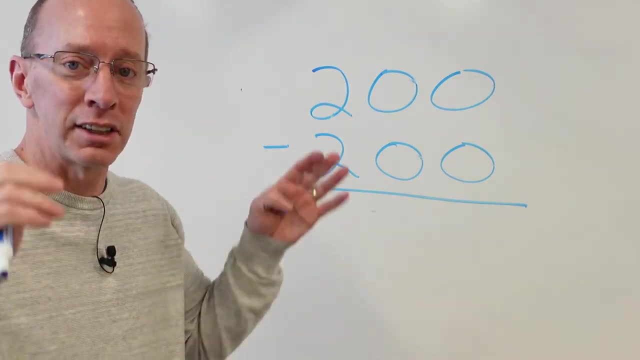 All right, Right away I can tell you math. ninjas, you are looking at this right in here, aren't you? Two minus two. Now don't get too confused. You know what. two minus two is right, You have something that is two. Two pieces of candy, two cars, two balls, two toys, something. 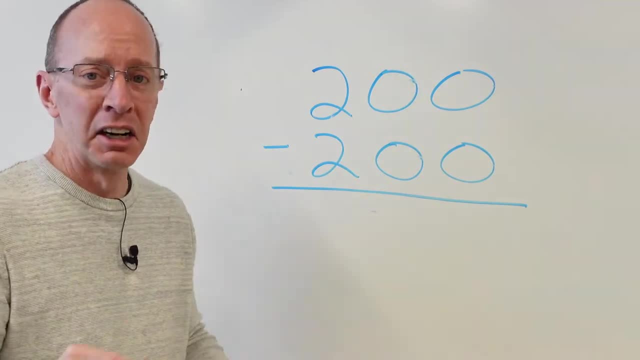 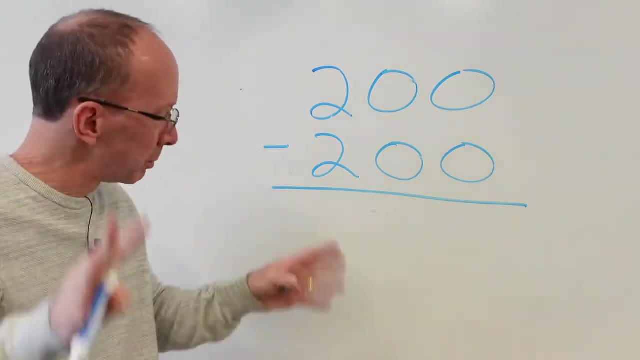 And you're taking away those. Maybe you had two pieces of candy and your younger brother took away the other two pieces. I don't know. You don't have anything. Okay, I'm sorry, It's in the past. In the past, Let's move on. 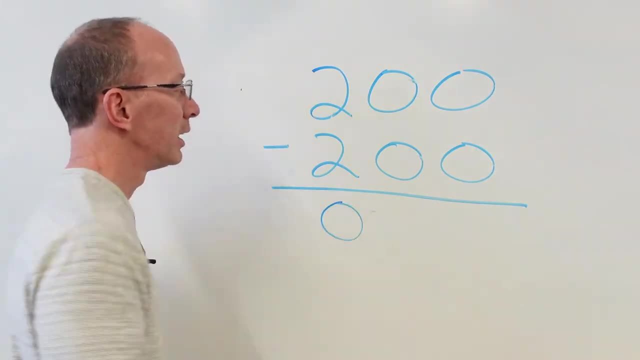 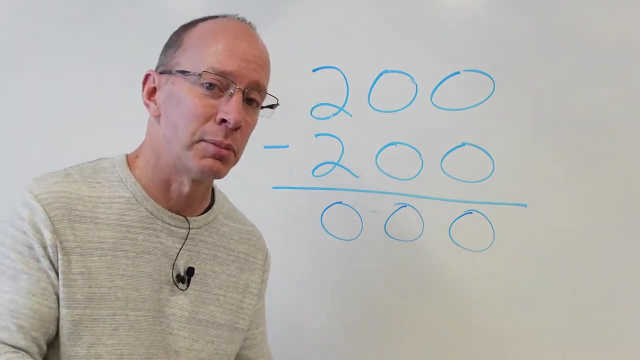 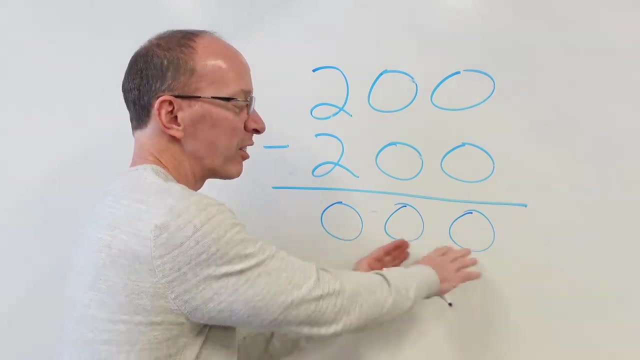 So two minus two is zero. All right, Drop down the other one, Zero. Drop down the other one Zero. Now you can talk to your teacher about this, But for the original answer, you don't really want to give all these zeros right here, Okay? 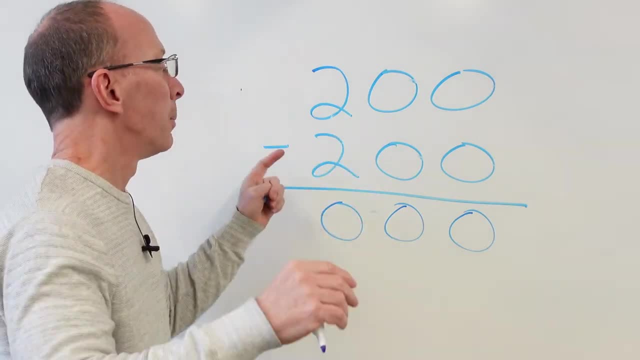 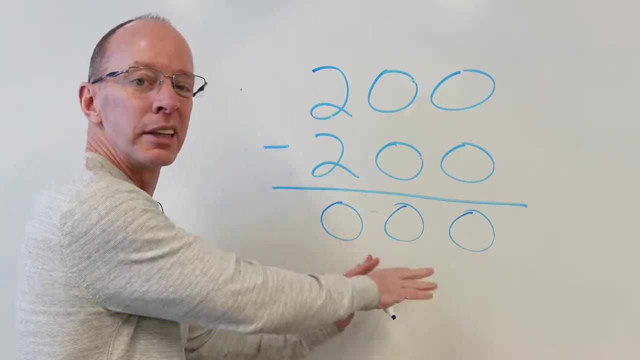 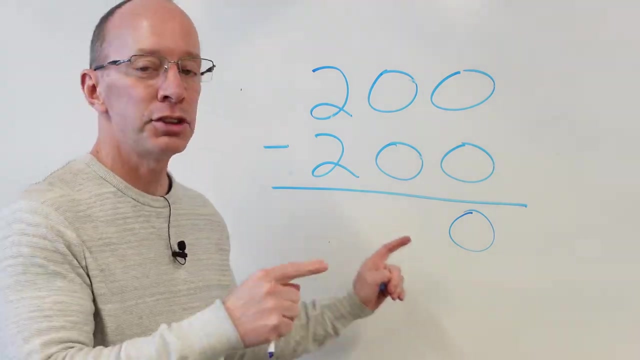 You want to take. you don't want to say: 200 minus 200 is zero, zero, zero, No, All right. So you kind of want to erase some of these zeros here. Right there, 200 minus 200 is zero. 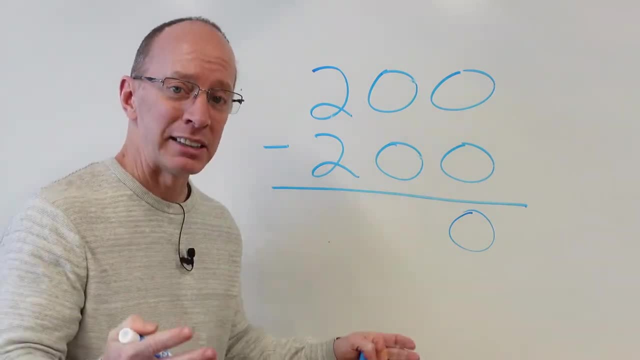 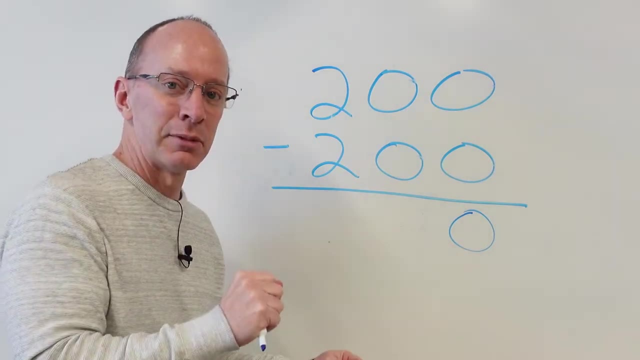 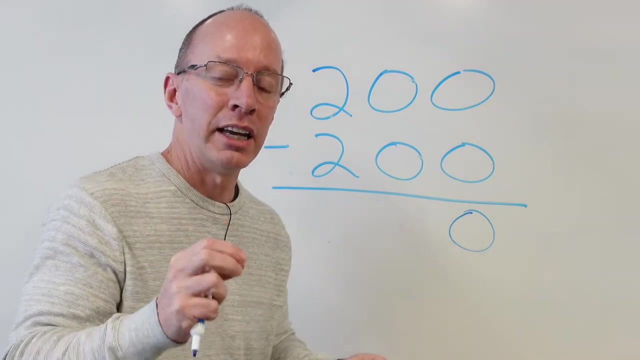 Now this is a challenging problem because I've, as being a teacher, I've seen a simple problem like that kind of be a little bit of a hiccup, kind of be of a challenge for some of my students. But I tell them that 200 minus 200 is zero. It would be like if I told you if you had one. 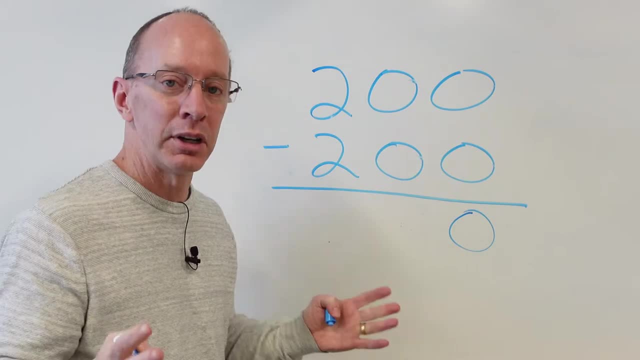 million dollars in your pocket. you would have a million dollars in your pocket. You would have a million pieces of candy. I don't know why you would have one million pieces of candy, But if you had one million pieces of candy and your younger brother took away one million pieces of, 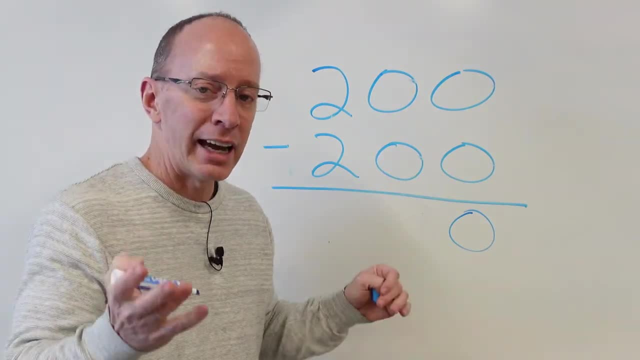 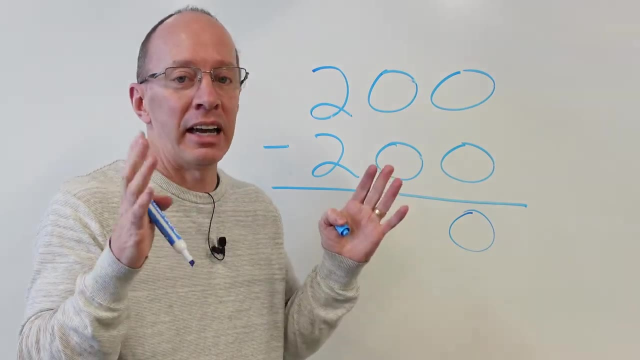 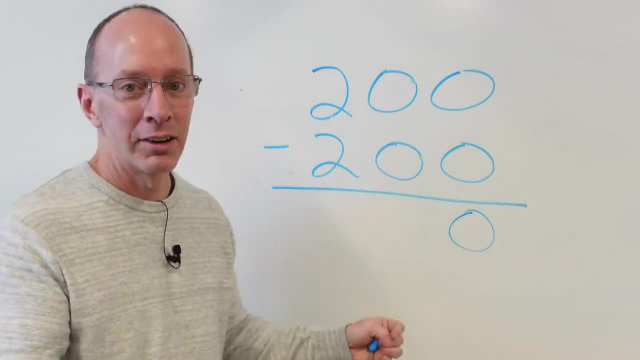 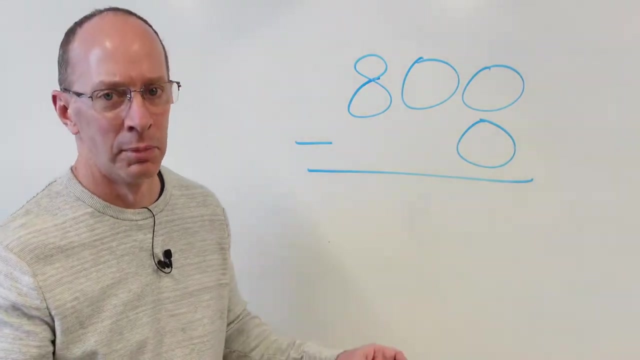 So 200 minus 200 is zero. Okay, Let's do the other. another problem: All right, Let's do it. Yeah, Do it. Boom, Here we go. You're saying, oh, come on, You're giving us. 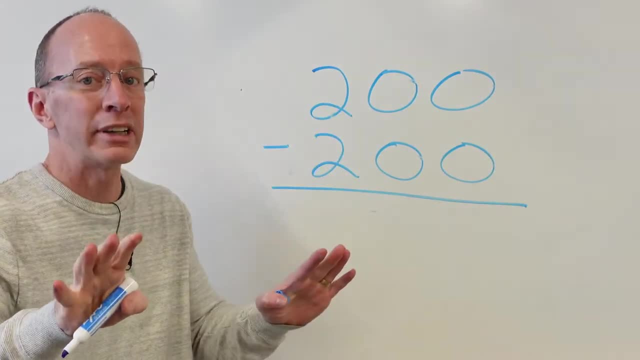 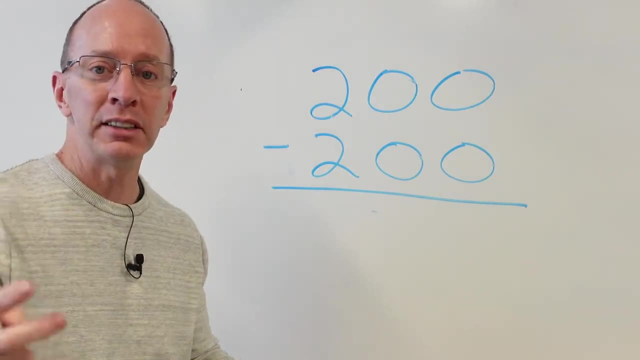 right in here, aren't you? Two minus two. Now, don't get too confused. You know what two minus two is. right, You have something that is two: Two pieces of candy, two cars, two balls, two toys. 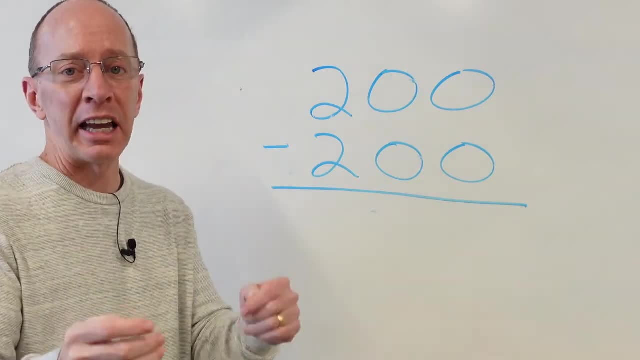 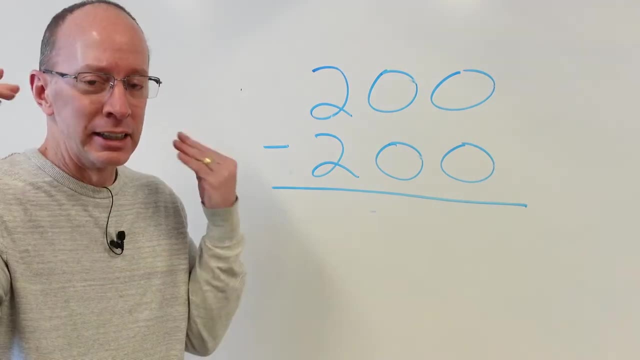 something And you're taking away those. Maybe you had two pieces of candy and your younger brother took away the other two pieces. I don't know. You don't have anything. Okay, I'm sorry. In the past, In the past, Let's move on. So two minus two is zero. All right, Drop down the other. 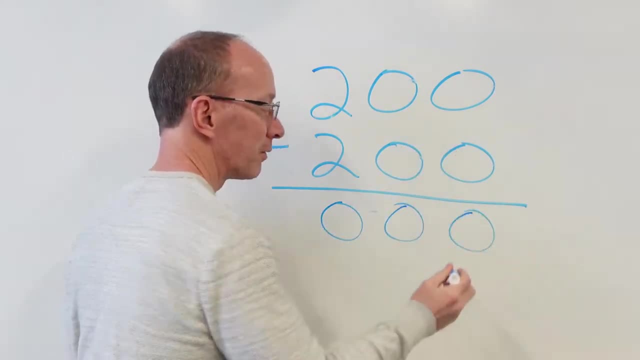 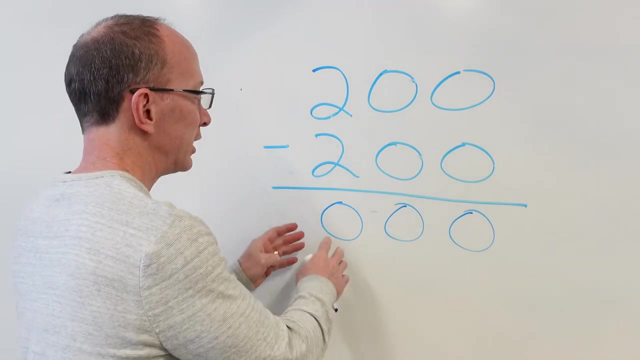 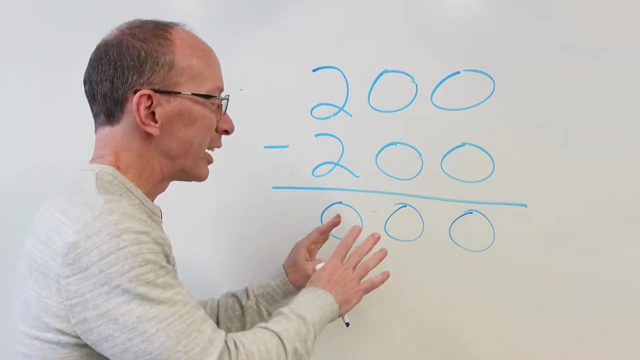 one Zero, Drop down the other one, Zero. Now you can talk to your teacher about this, But for the original answer you don't really want to give all these zeros right here. Okay, You want to take. you don't want to say 200 minus 200 is zero, zero, zero. 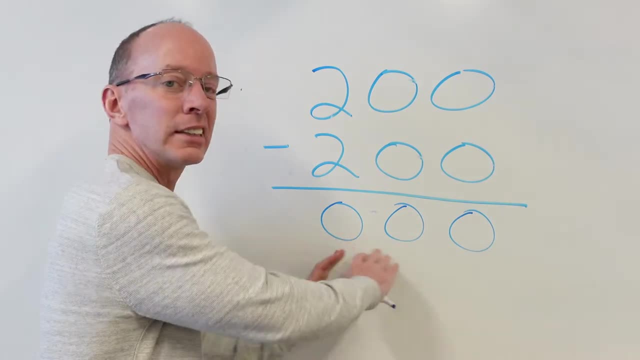 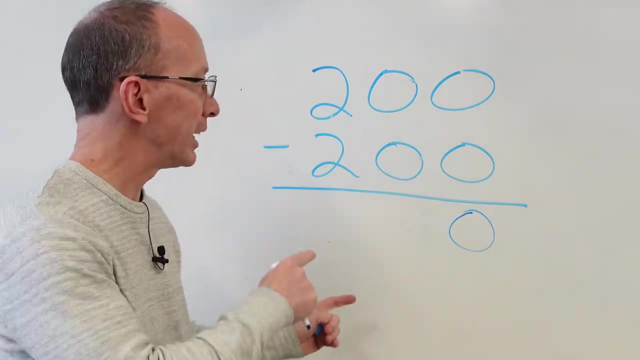 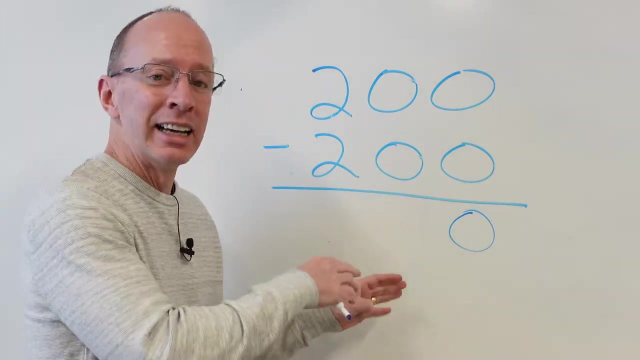 No, All right, So you kind of want to erase some of these zeros here, Right there, 200 minus 200 is zero. Now this is a challenging problem because I've, as being a teacher, I've seen a simple problem like that kind of be a little bit of a hiccup. 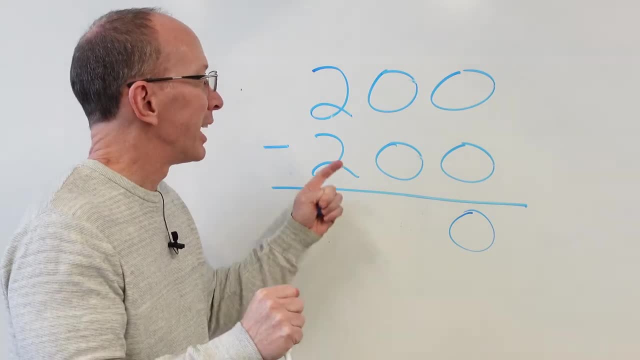 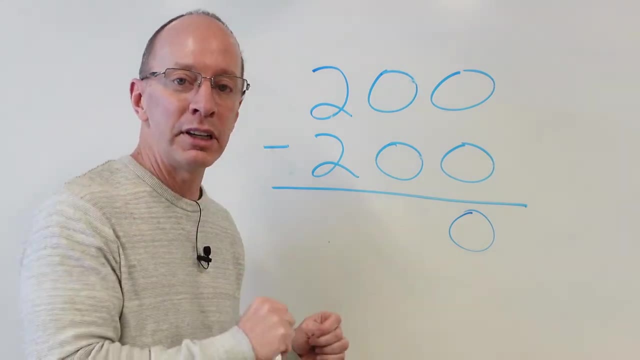 kind of be of a challenge for some of my students. But I tell them that 200 minus 200 is zero. It is zero, Okay. So if you had one million pieces of candy, I don't know why you would have one. 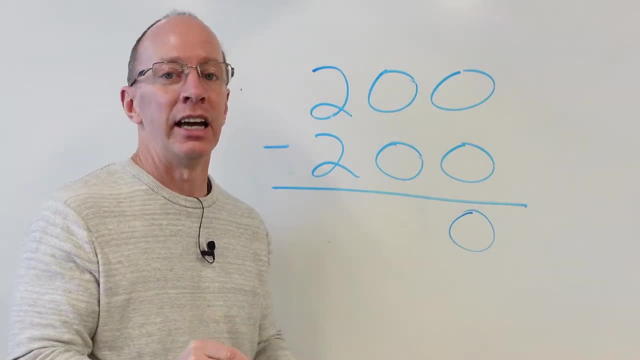 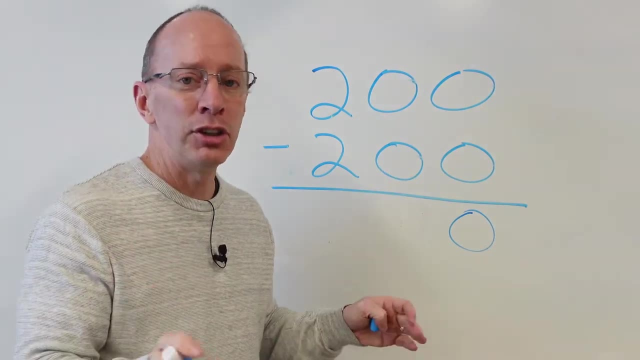 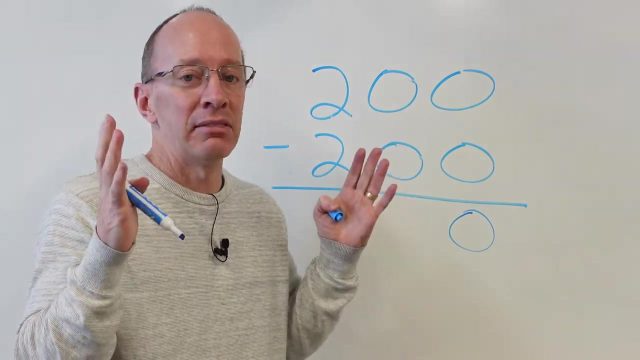 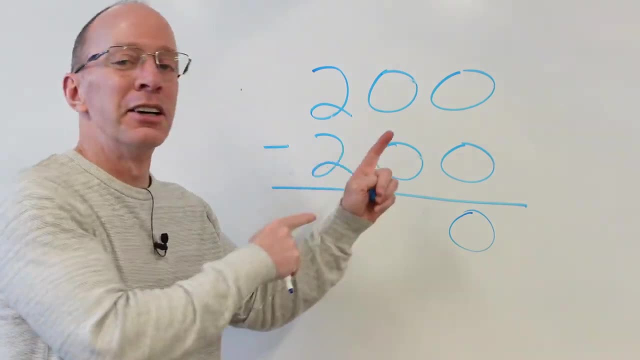 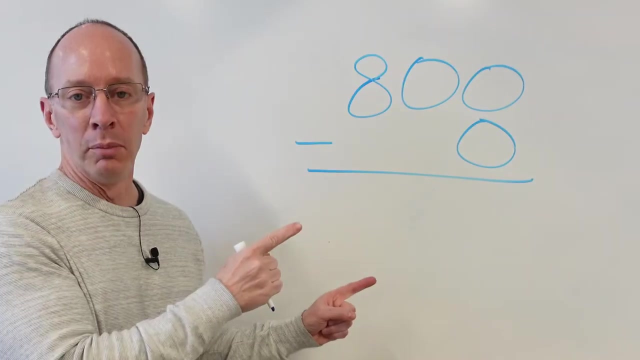 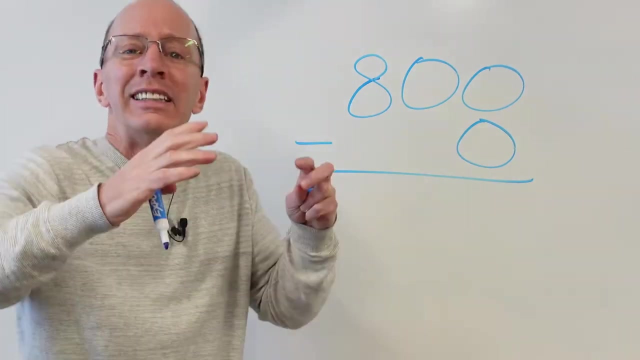 nothing, All right. So 200 minus 200 is zero. Okay, Let's do the other. another problem: All right, Let's do it. Yeah, Do it. Boom. Here we go. You're saying, oh, come on, You're giving us challenging problems all the time. No, Take it. 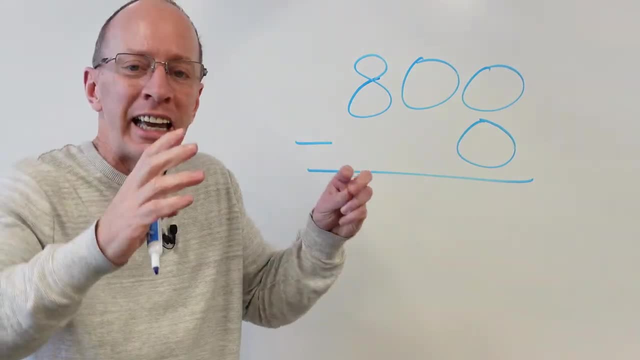 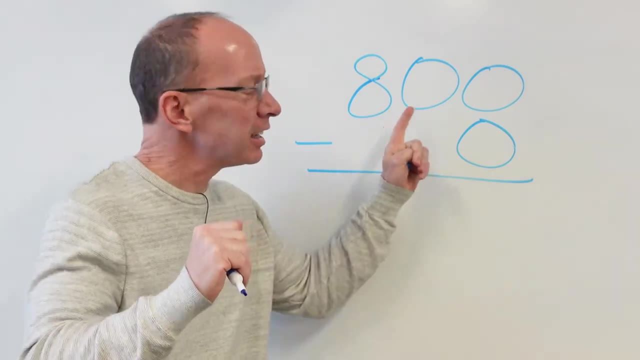 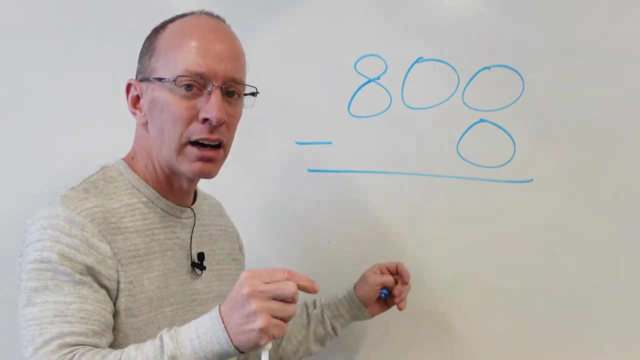 challenging problems all the time. No, Take it a little at a time. Take a little time and baby steps. All right, You got 800 minus zero. Think about that. All right, You have 800 minus zero. That means let's back it up, Let's say you have an apple. 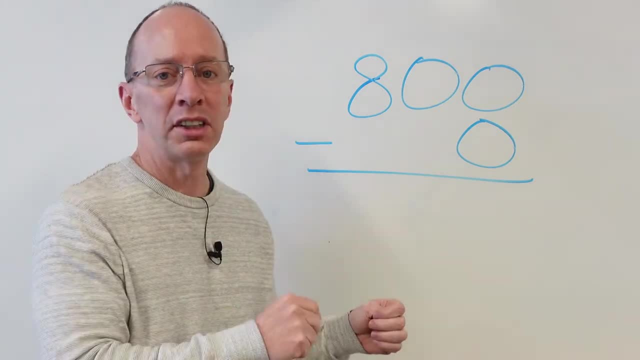 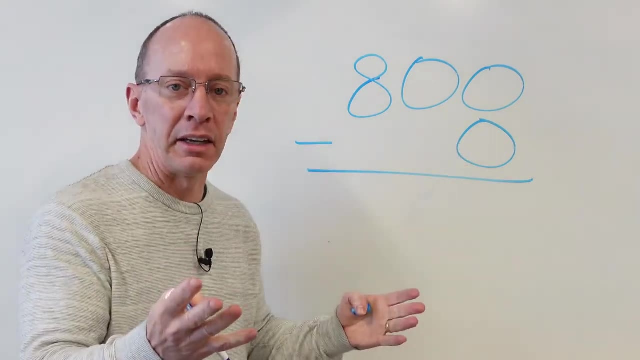 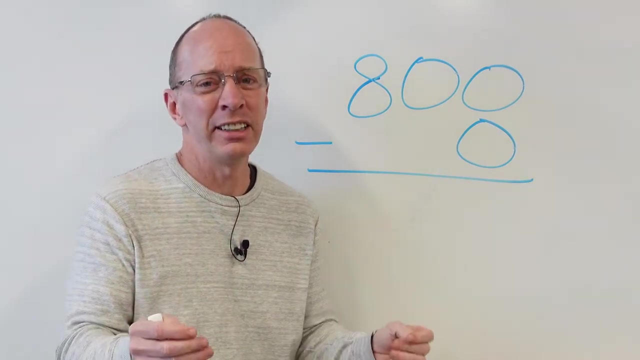 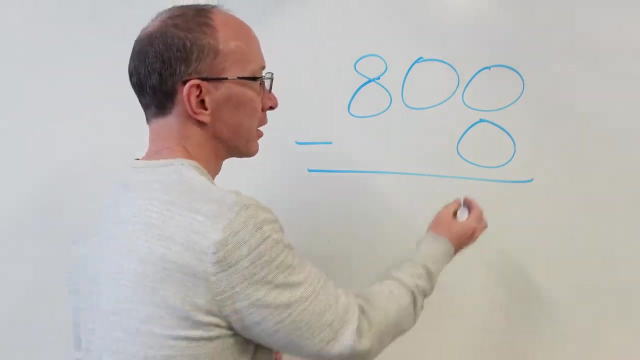 All right, And no one took it away. You still have that apple. You have 800 pieces of candy and your little brother didn't take any of it away. All right, So how many do you have? Tell me? tell me, How many do you have? 800 minus zero, is you still got 800.? Okay, You drop it down. 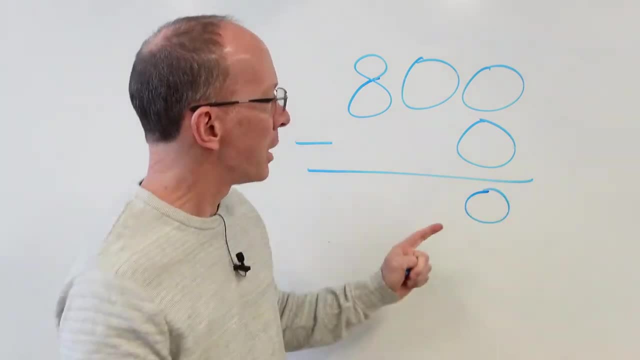 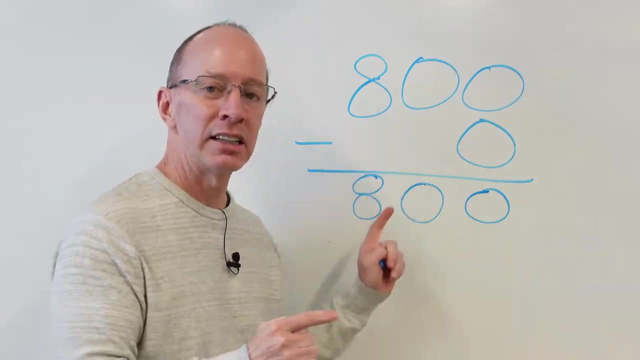 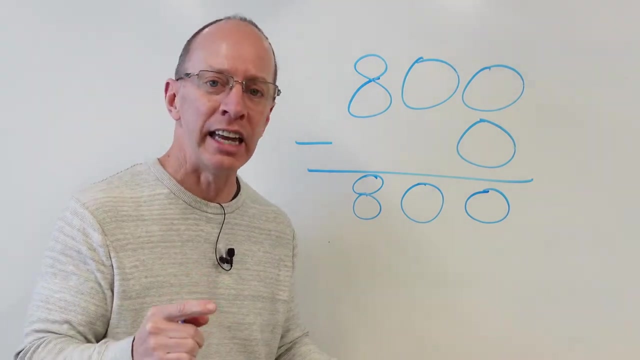 You drop it down. Yeah, Zero, Boom. You drop the zero down, Boom. You drop the eight down, You got 800.. 800 minus zero is 800.. You should be happier than a dog with two tails because you still got your 800 pieces of candy. Oh, yeah, All. 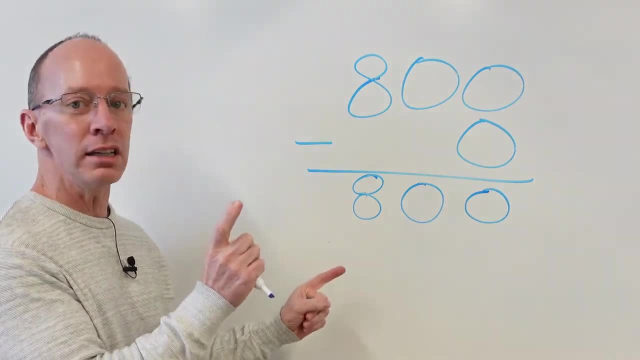 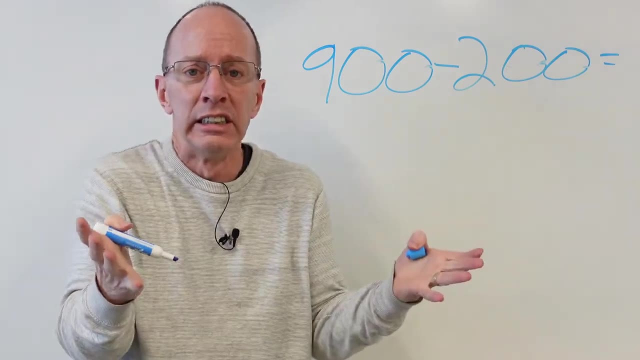 right, Let's go on to the next problem. You ready? All right, Let's do it. Boom There it is 900 minus 200.. You're saying, oh, this is written differently, Don't worry, All you have to do is: 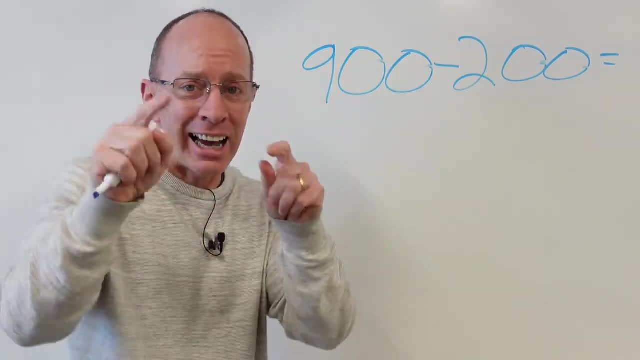 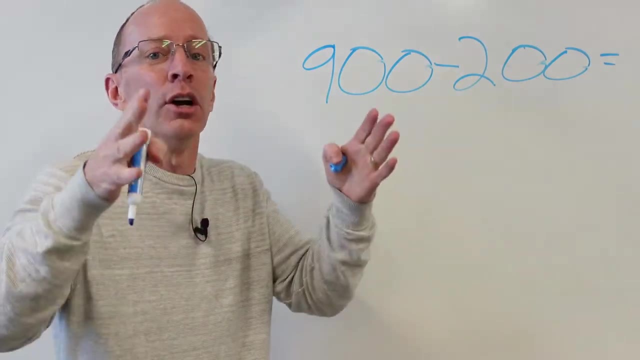 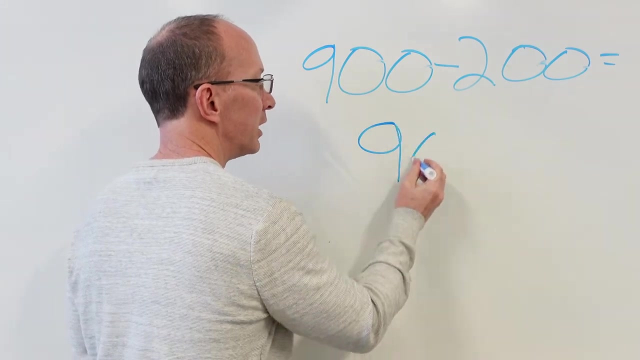 rewrite it. All right, I got going over rewriting in another video. Check out my other math videos. on here I go more in depth on how to rewrite a number, All right. So basically you just take this number right here: Okay, Put it right here: 900.. Then you write the other number down below it. 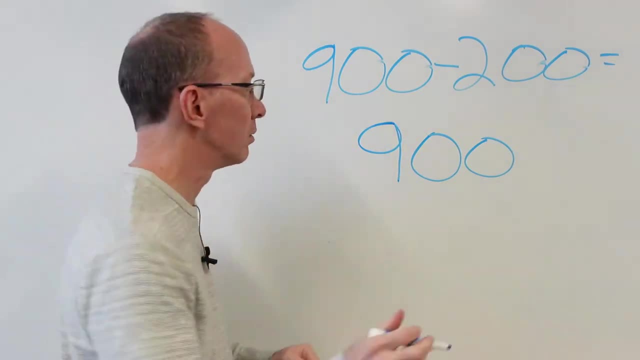 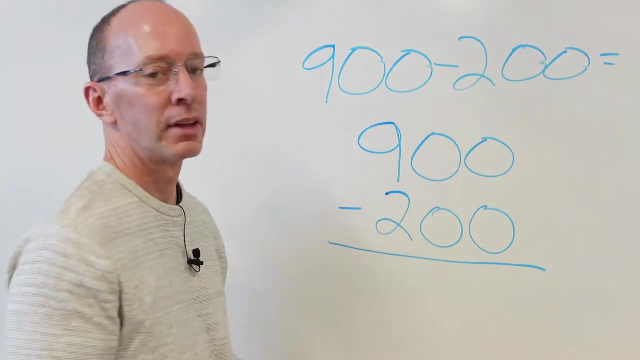 Make sure you line up your hundreds, your tens and your ones. So I put a two right here, another zero, another zero. Put a little subtraction line right there. Now, this is going to be on paper, but I just don't. 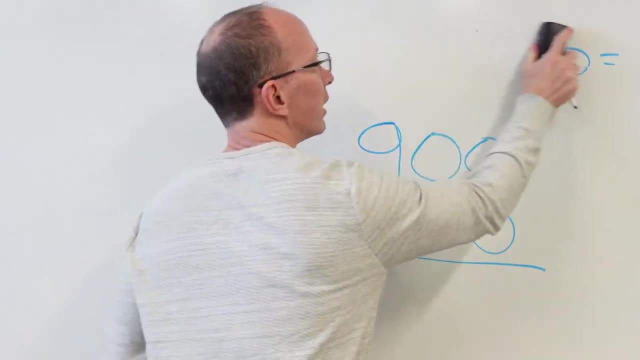 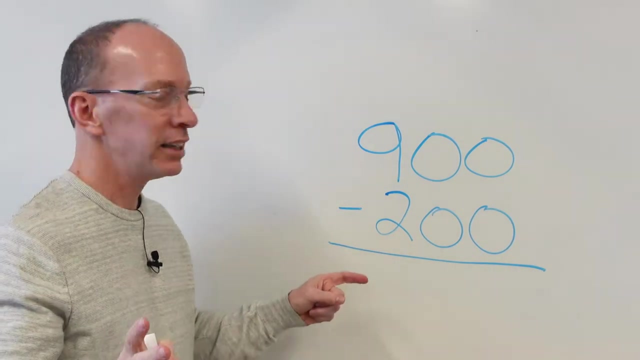 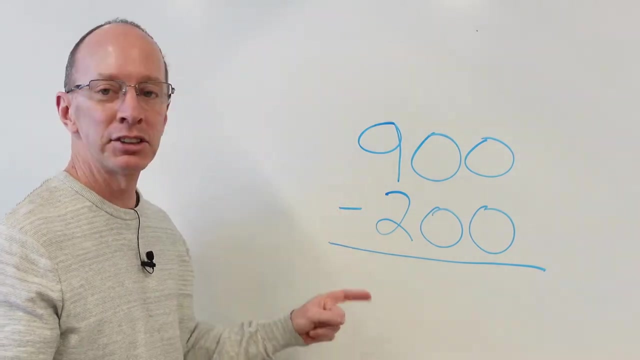 want to get that confusing, So I'm just going to erase that part right there so we can concentrate on this Right away. where are your eyes focusing? Where are they? Yes, They are focusing on the nine minus two, aren't they? You betcha? All right, Nine minus two, What is it? Seven, seven, eight. 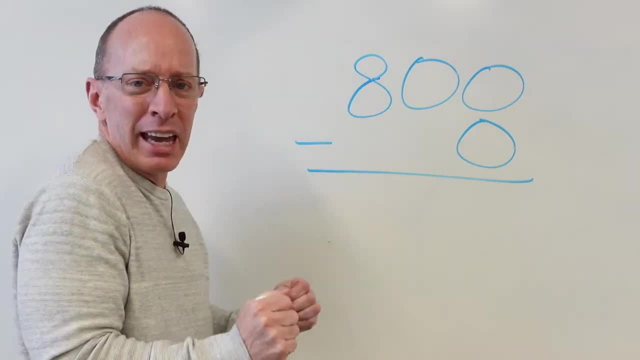 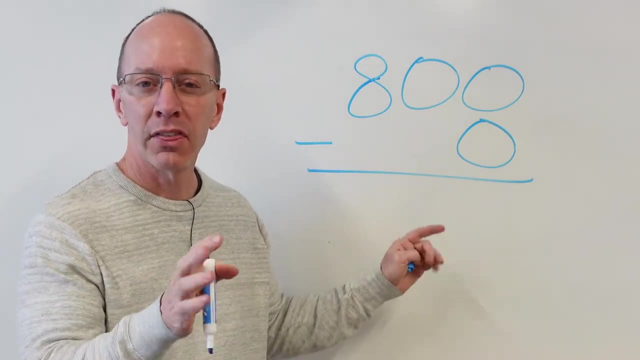 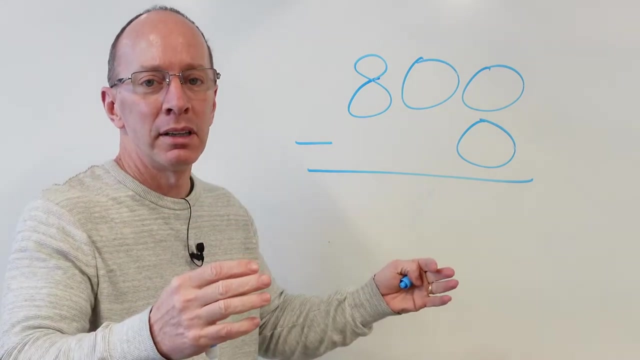 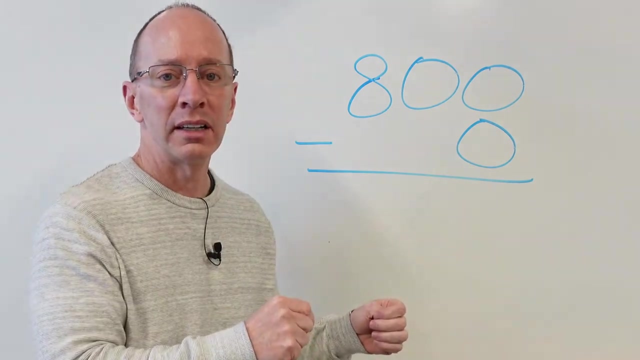 little at a time, Take little time and baby steps. All right, You got 800 minus zero. Think about that. All right, You have 800 minus zero. That means let's back it up. Let's say you have an apple. All right, And no one took it away, You still have that apple. You have 800. 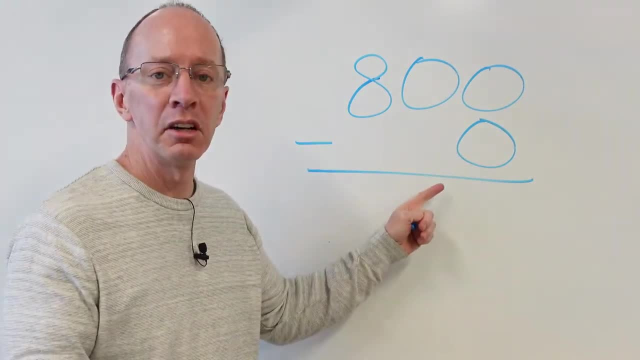 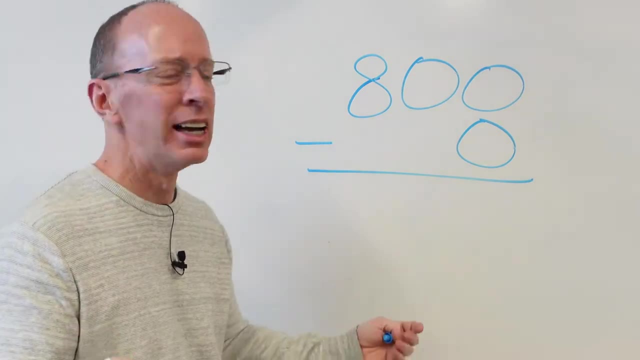 pieces of candy and your little brother didn't take any of it away. All right, So how many do you have, Tell me? Tell me, How many do you have? 800 minus zero, is you still got 800. Okay, You. 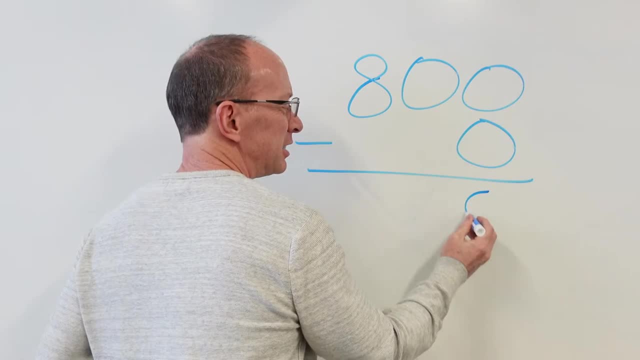 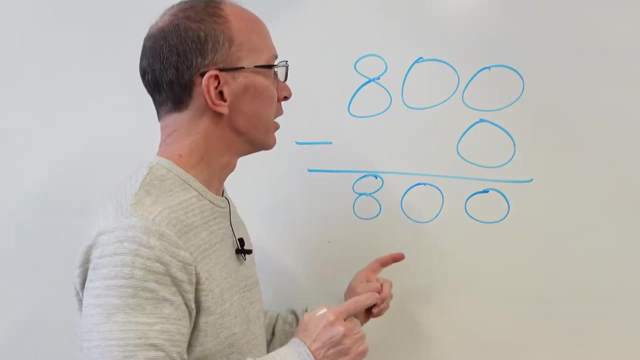 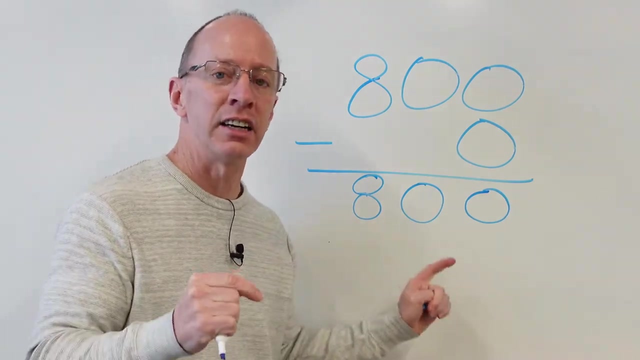 drop it down, You drop it down, Yeah, Zero, Boom. You drop the zero down, Boom. You drop the eight down, You got 800.. 800 minus zero is 800. You should be happier than a dog with two tails, because you still got your 800 pieces of. 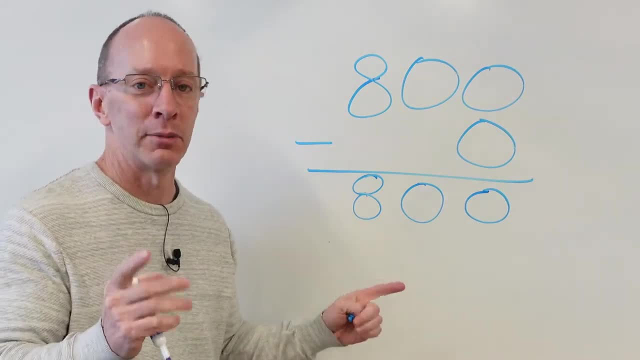 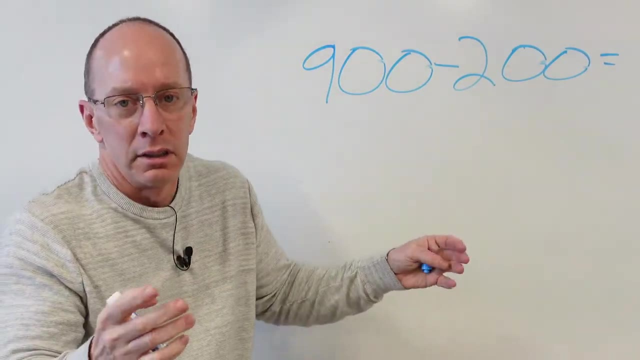 candy. Oh yeah, All right, Let's go on to the next problem. You ready? All right, Let's do it. Boom There, it is 900 minus 200.. You're saying, oh, this is written differently. 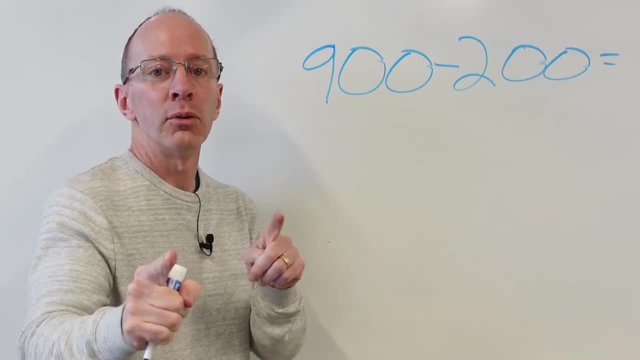 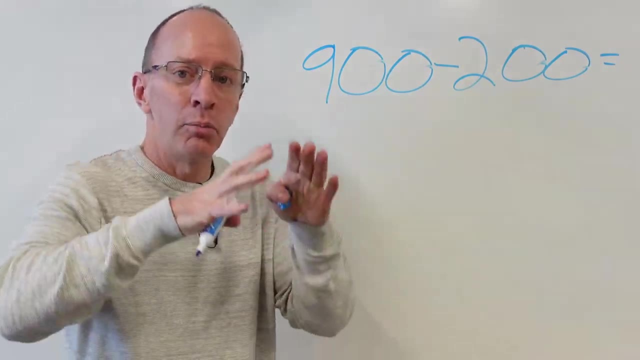 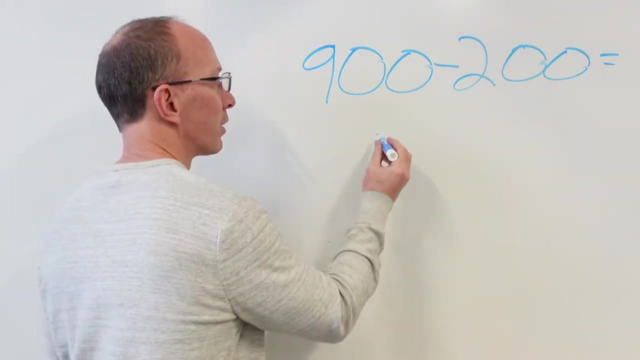 Don't worry, All you have to do is rewrite it. All right, I got going over rewriting in another video. Check out my other math videos on here. I go more in depth on how to rewrite a number, All right. So basically you just take this number right here. Okay, Put it right here: 900.. 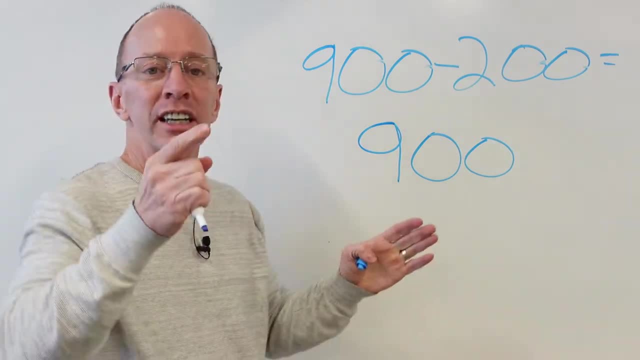 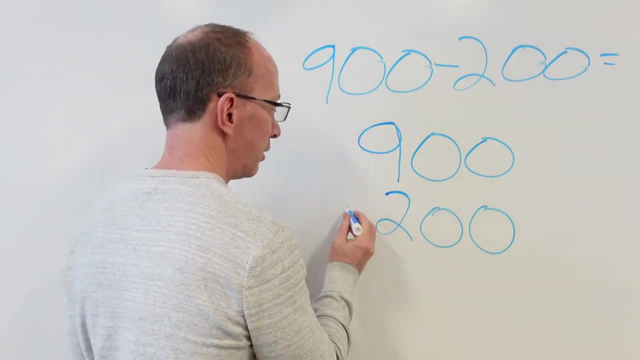 Then you write the other number down below it. Make sure you line up your hundreds, your tens and your ones. So I put a two right here, Another zero, Another zero. Put a little subtraction line right there. Now this is going. 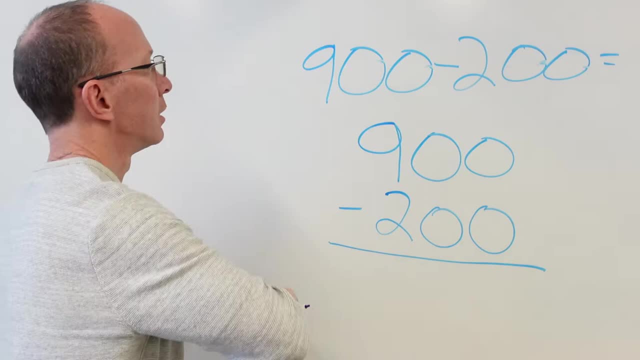 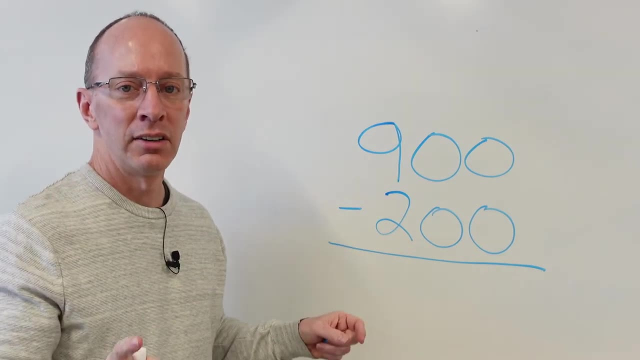 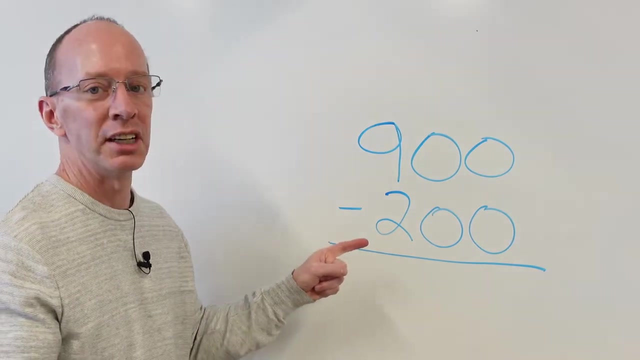 to be on paper, but I just don't want to get that confusing, So I'm just going to erase that part right there so we can concentrate on this Right away. where are your eyes focusing? Where are they? Yes, They are focusing on the nine minus two, aren't they? You betcha, All right, Nine. 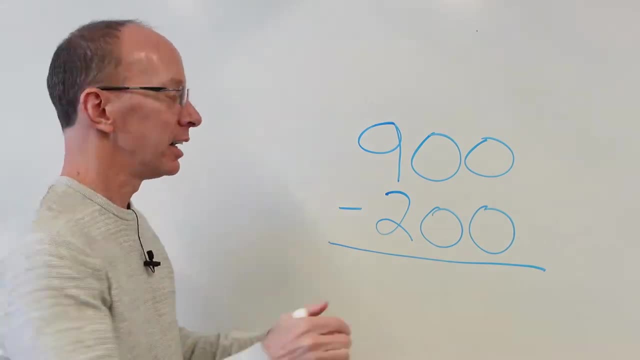 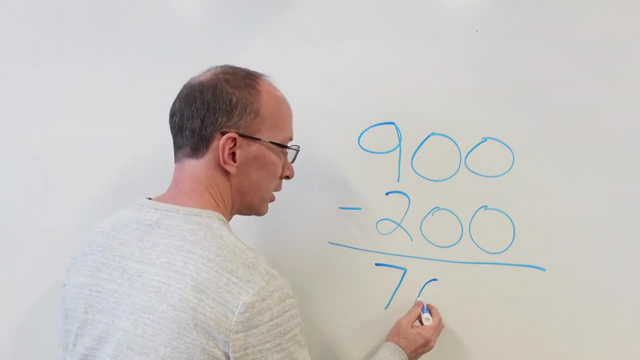 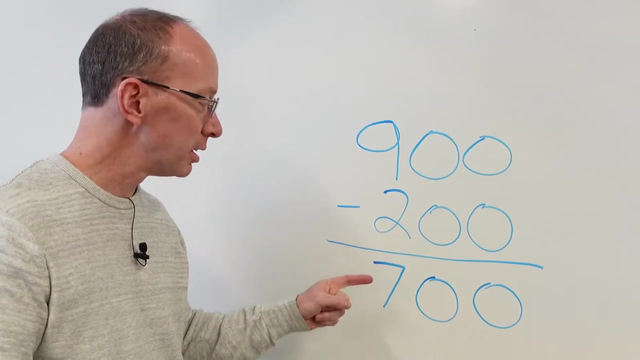 minus two, What is it? Seven, Seven, Eight, Nine, It is seven, Sent from heaven. Okay, So then we drop down the zeros. Okay, Put a zero here. We put a zero here. That gives us 900 minus two. 900 minus 200 is 700. All right Now, if you want to, I don't know if- 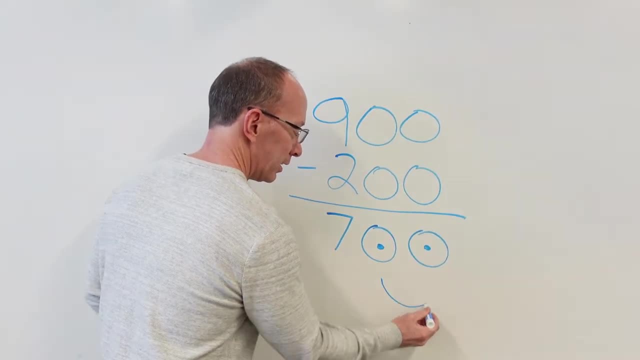 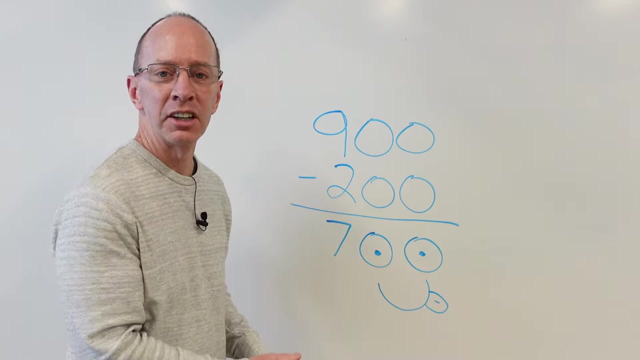 your teacher will allow you. You can always put a little dot here, a little dot here and a little smiley face with a tongue sticking out there. Okay, Maybe that was a bad idea, but it kind of looks, kind of cute. Okay, Are you ready to do a story problem? 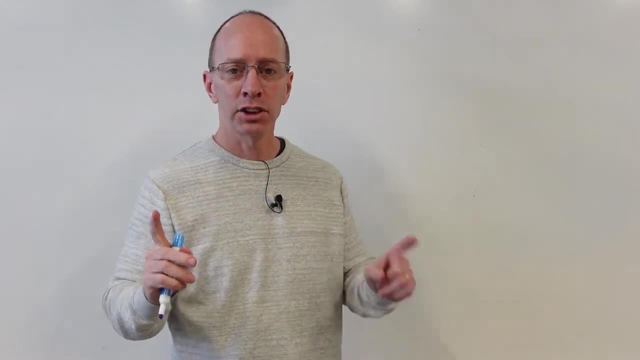 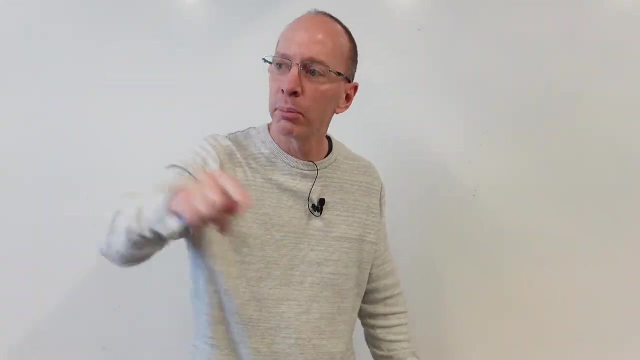 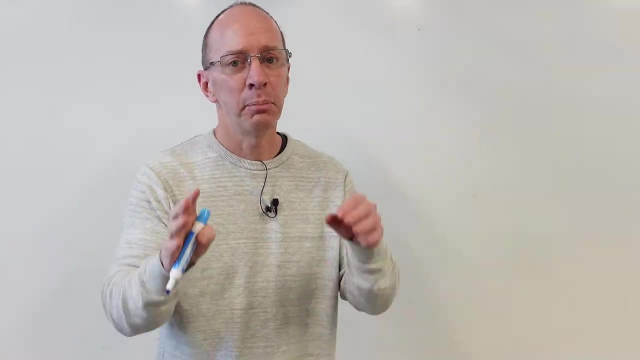 Yeah, Let's do it. Boom, Okay, Here is our story. problem of the day: You have 600 bananas. Yes, I know that they're your bananas. Oh, my goodness gracious, Settle down. I'll give you the bananas after class. Okay, There are 600 bananas, but then the cows came over and took. 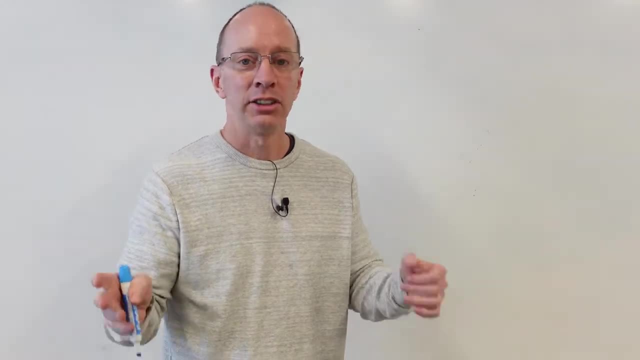 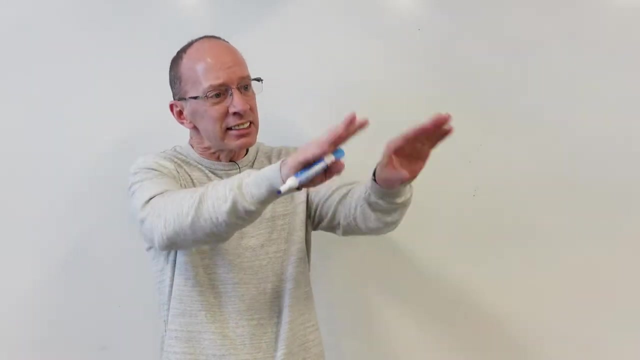 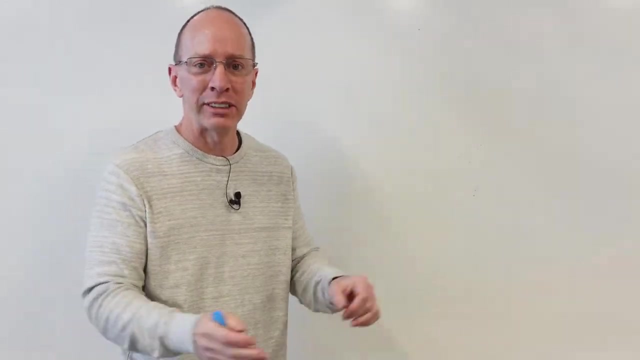 200.. I don't know why cows would take 200 bananas, but I need to know how many more bananas are left for the monkey. Yes, Yes, yes, yes, We'll get you the banana, And I don't know why the cows took the 200 bananas. Maybe this was a different. maybe I could have chose a different. 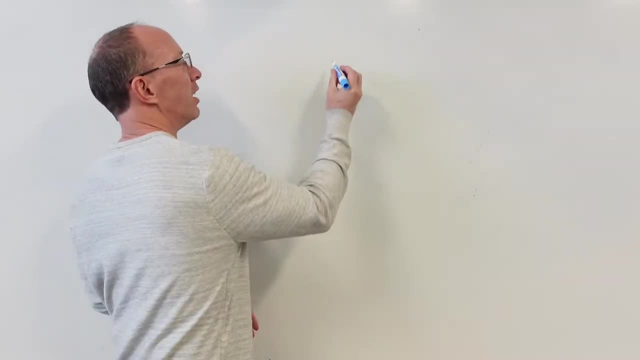 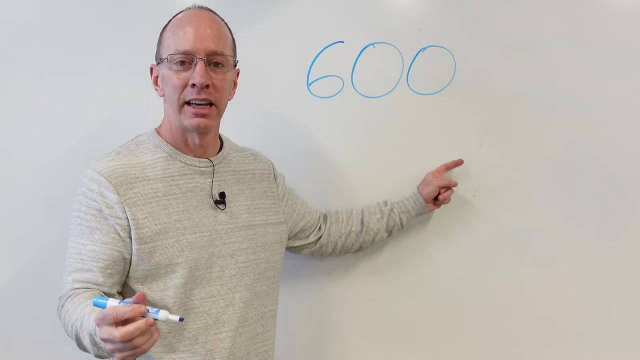 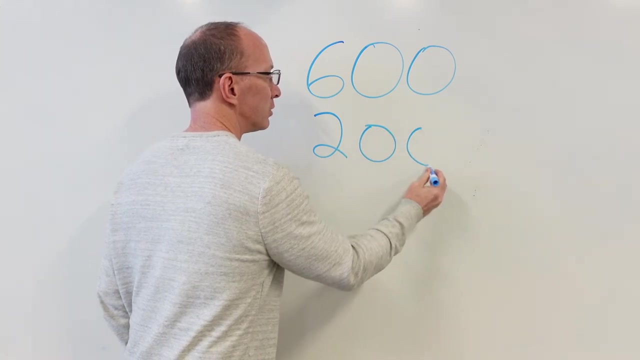 story problem, But anyway, let's just continue. Let's go on. All right, We have 600 right here. That represents the 600 bananas. Now the cows took away 200 of those bananas. Okay, So I write down 200 right here and this is the bananas. 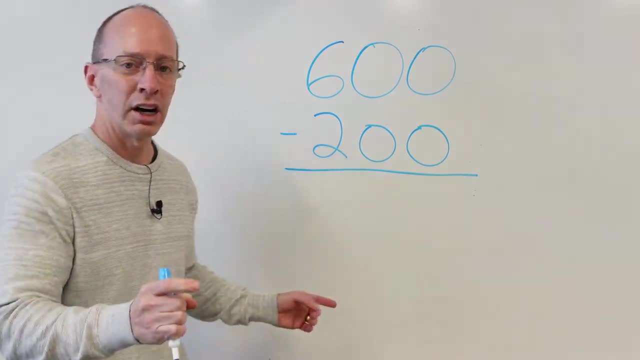 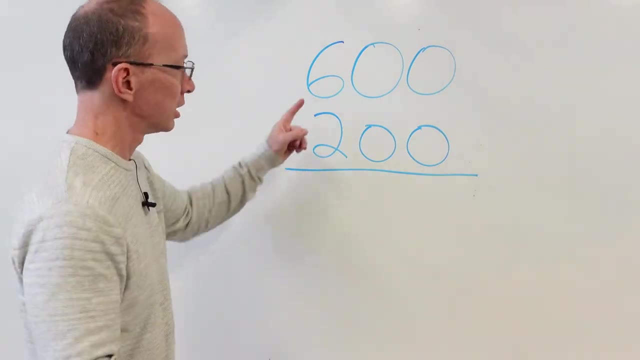 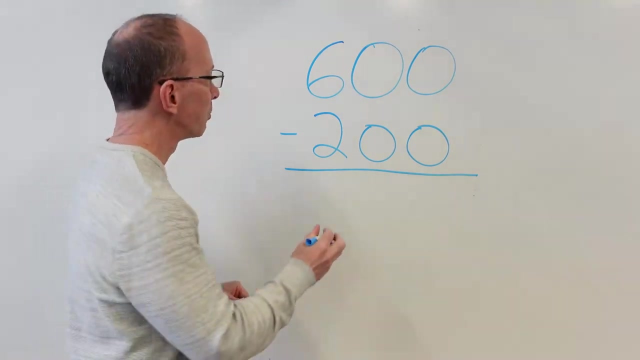 This is going to be a subtraction problem. Okay, Where are your ninja eyeballs looking at? Boom, Right there. Six minus two, Yeah, Six minus two is what? Uno, dos, tres, cuatro, Always throwing in a little Spanish with my lesson here. Four, Drop down the zero. 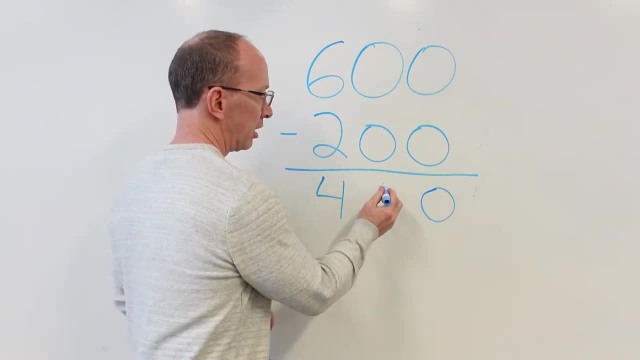 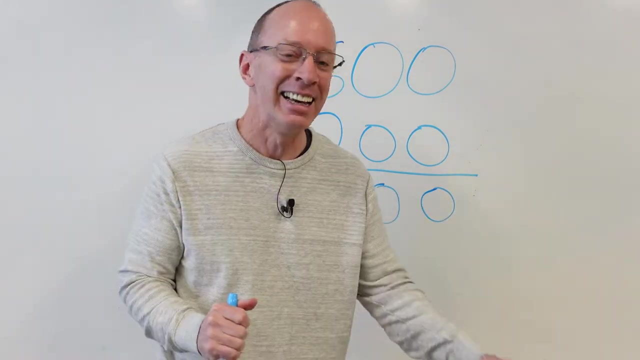 You drop down the zero, You drop it down, Drop it down, Drop down the zero, Drop down the zero. I'm doing it. The moonwalk You can't tell. Drop down the zero, Okay. So how many bananas do we have left? 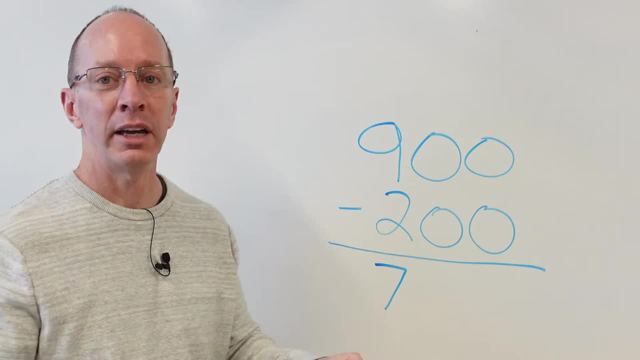 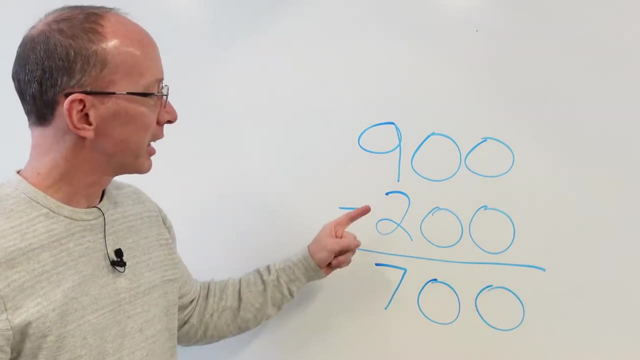 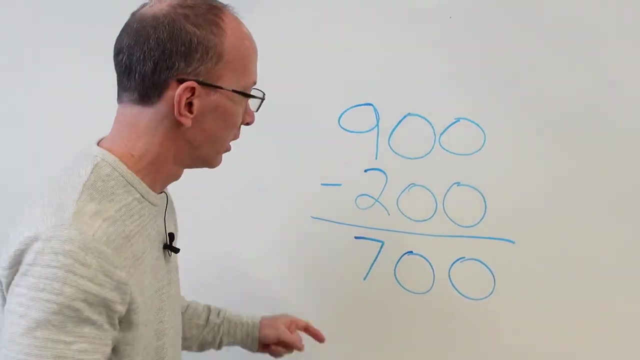 nine, It is seven, sent from heaven. Okay, So then we drop down the zeros. Okay, Put a zero here. We put a zero here. That gives us 900 minus two. 900 minus 200 is 700.. All right Now, if you want to. I don't know if your teacher will. 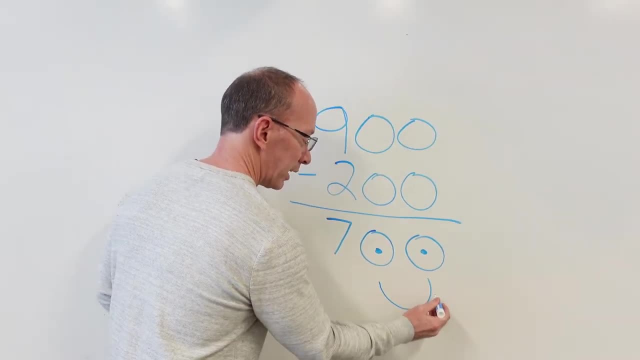 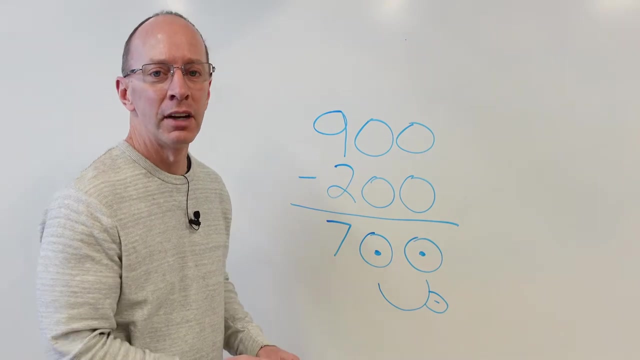 allow you, you can always put a little dot here, a little dot here and a little smiley face with a tongue sticking out there. Okay, Maybe that was a bad idea, but it kind of looks, kind of cute. Okay, Are you ready to do a story problem? Yeah, Let's do it Boom. 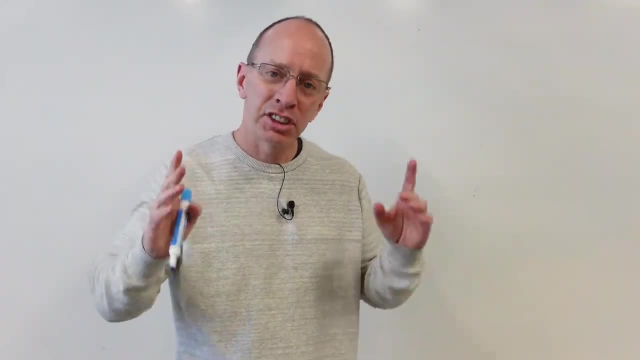 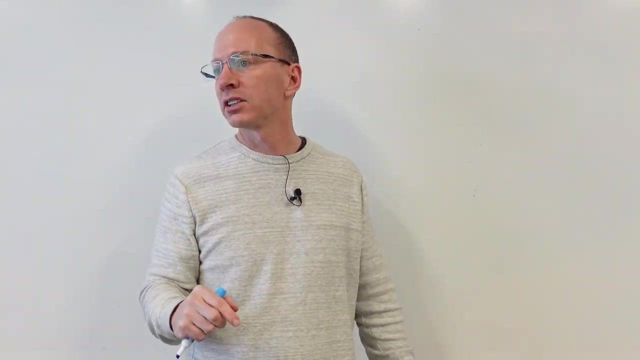 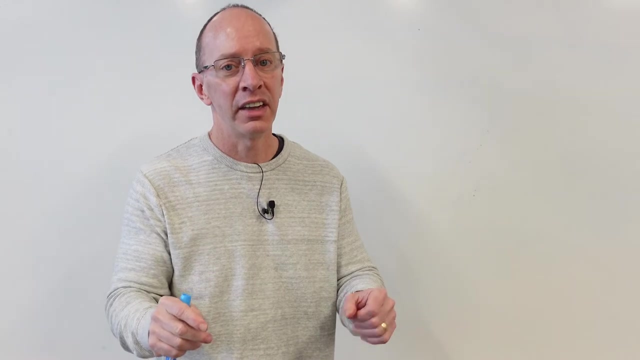 Okay, Here is our story problem of the day: You have 600 bananas. Yes, I know that they're your bananas. Oh, my goodness gracious, Settle down, I'll give you the bananas after class. Okay, There are 600 bananas, but then the cows came over and took 200.. I don't know why cows. 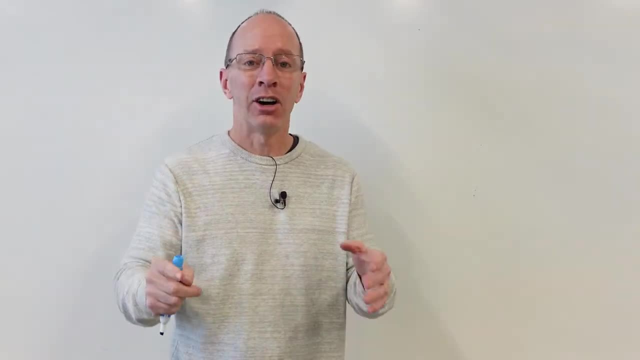 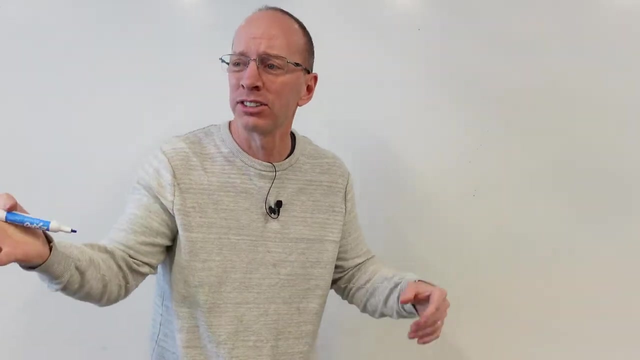 would take 200 bananas, but I need to know how many more bananas are left for the monkey. Yes, Yes, yes, yes, We'll get you the banana. And I don't know why the cows took the 200 bananas. Maybe this was a different, maybe I could have chose a different story problem, But anyway. 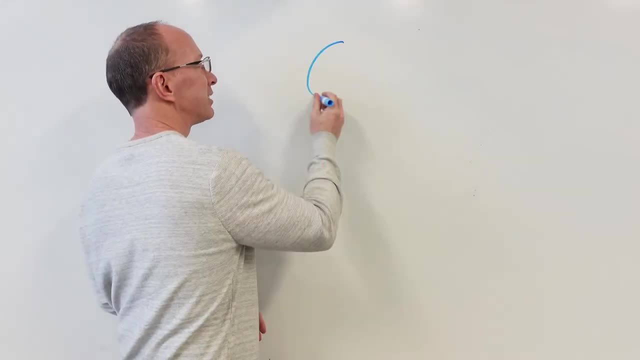 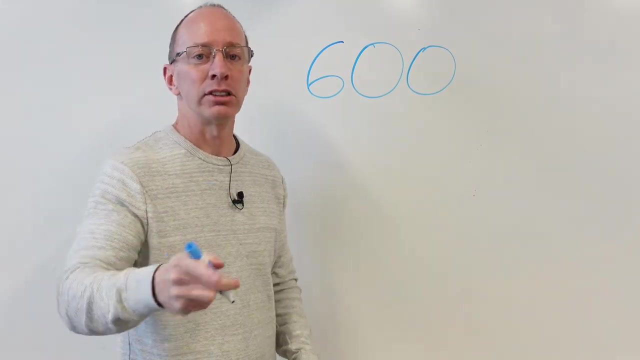 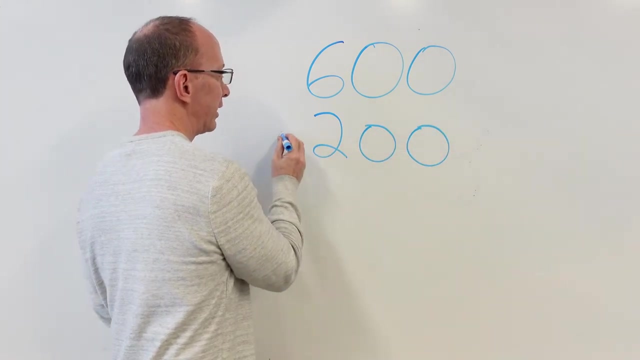 let's just continue. Let's go on. All right, We have 600 right here. That represents the 600 bananas. Now the cows took away 200 of those bananas. Okay, So I write down 200 right here and this is going to be a subtraction problem. 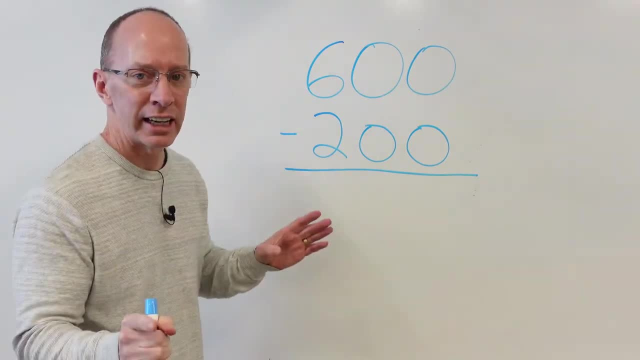 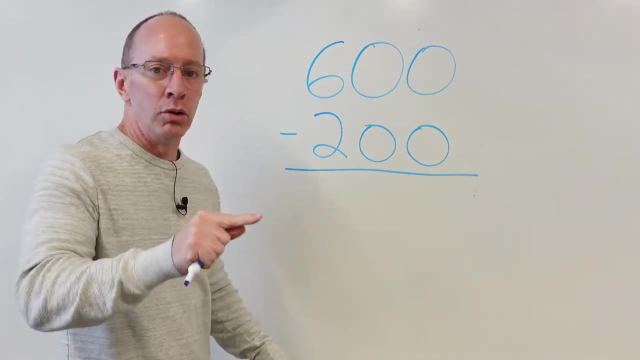 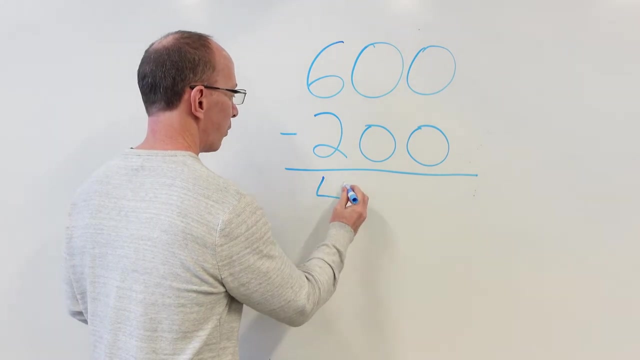 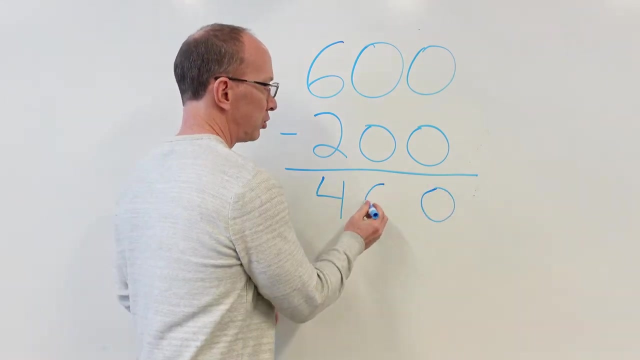 Okay, Where are your ninja eyeballs looking at? Boom, Right there. Six minus two. Yeah, Six minus two is what: Uno, dos, tres, cuatro, Always throwing in a little Spanish with my lesson here. Four: Drop down the zero. You drop down the zero. You drop it down, Drop it down. 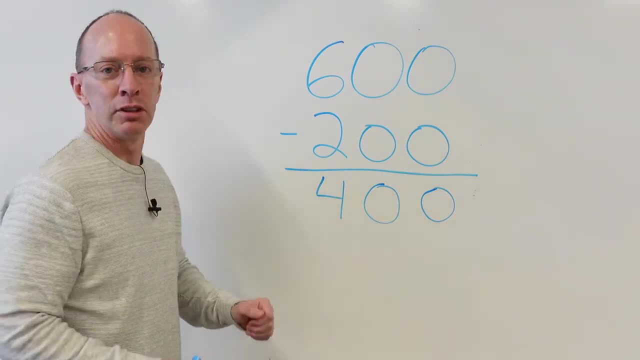 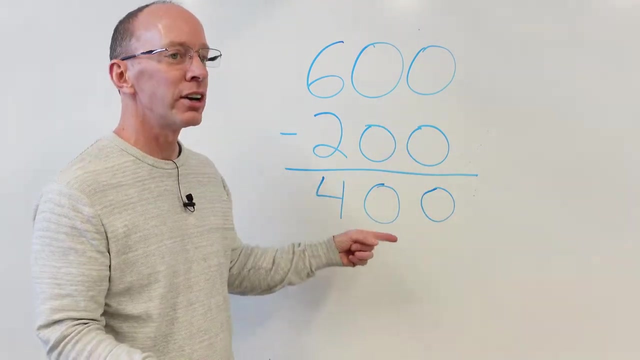 Drop down the zero. Drop down the zero. I'm doing the moonwalk, but you can't tell. Drop down the zero, Okay. So how many bananas do we have left? We have 400.. Yes, we have 400 bananas for you, monkeys.